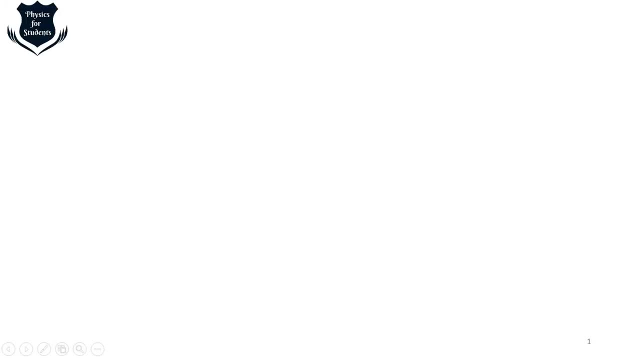 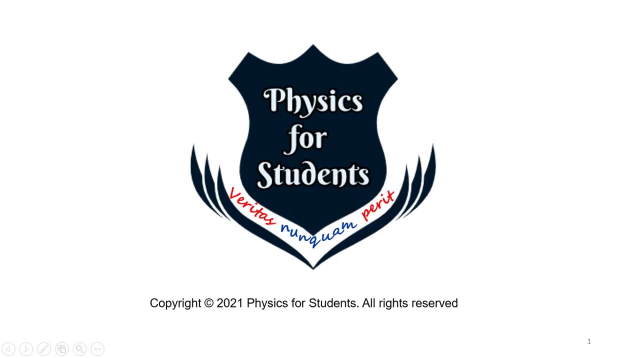 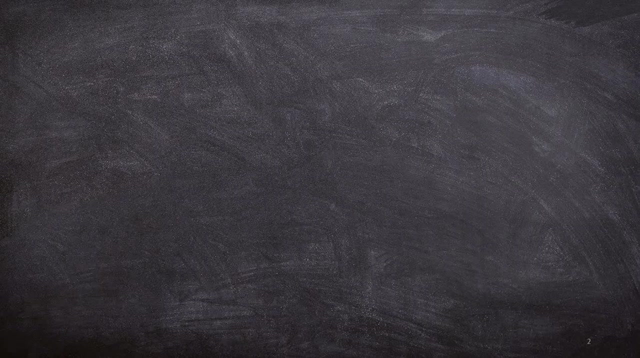 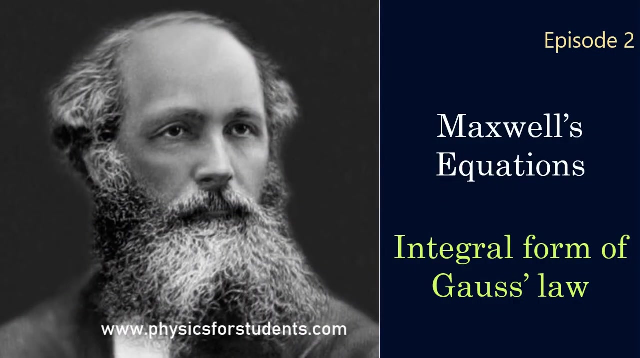 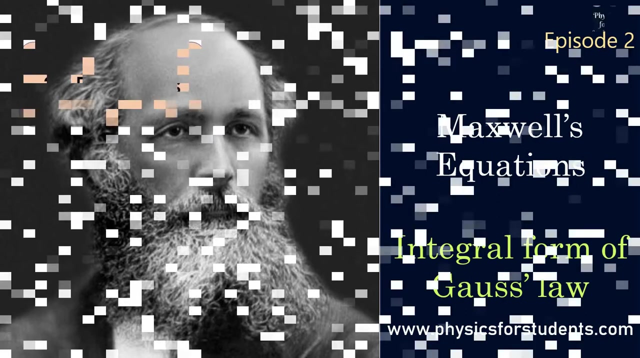 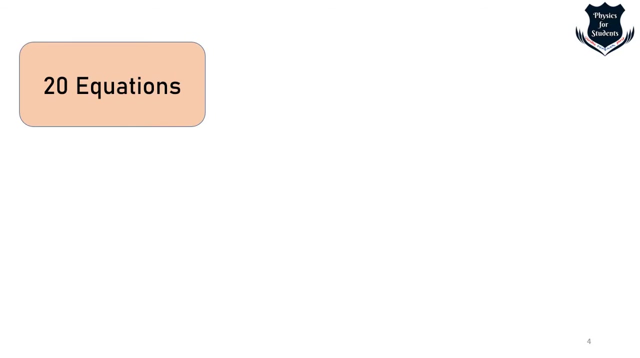 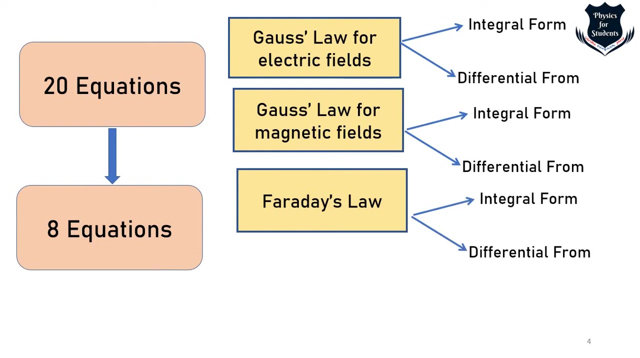 This video is presented to you by Physics for Students. To know more. please visit us at physicsforstudentscom To learn more. please visit us at physicsforstudentscom To learn more. please visit us at physicsforstudentscom To learn more. please visit us at physicsforstudentscom. 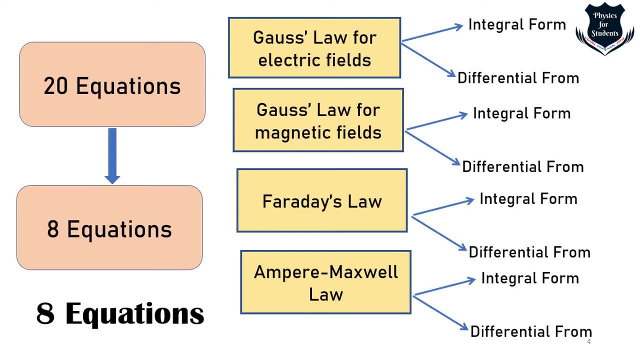 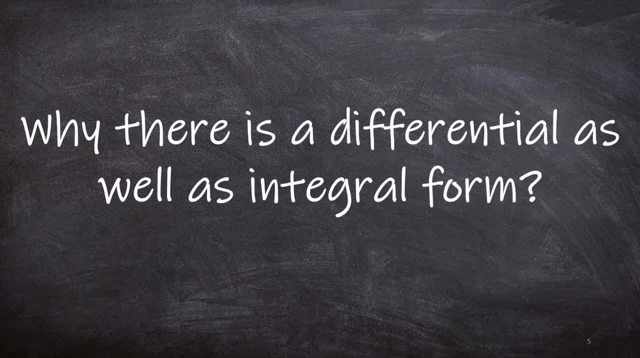 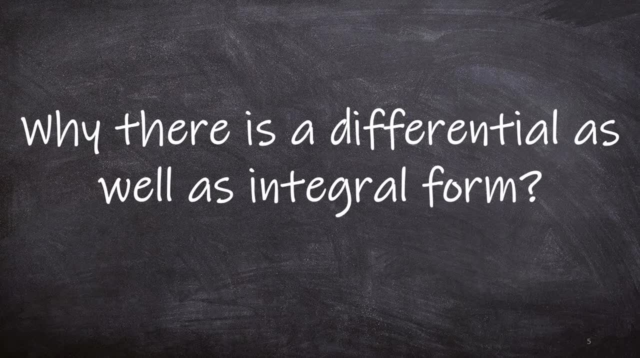 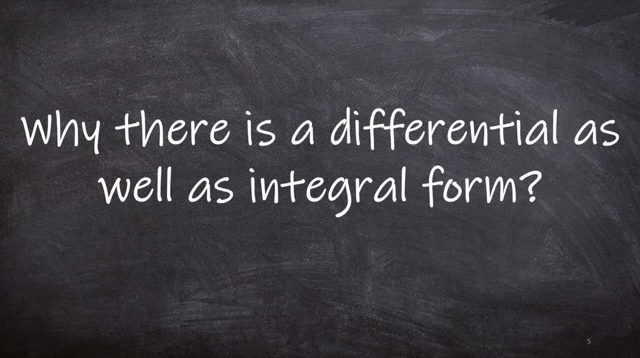 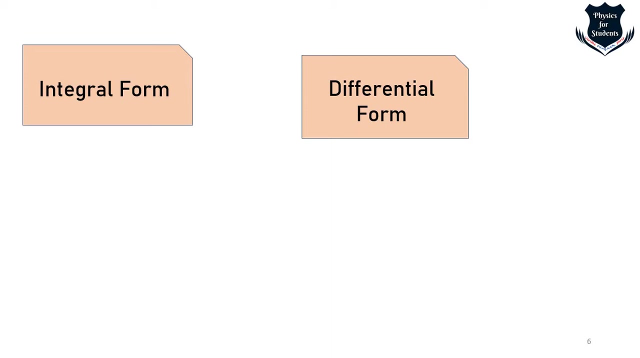 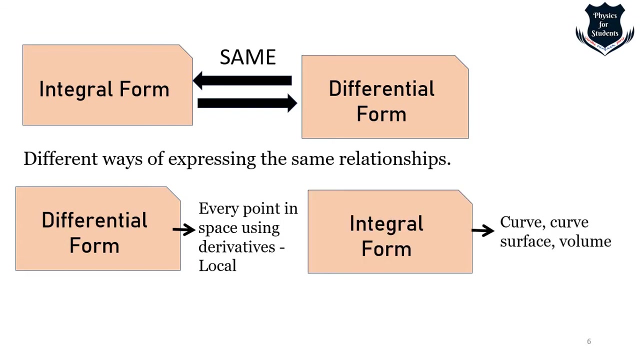 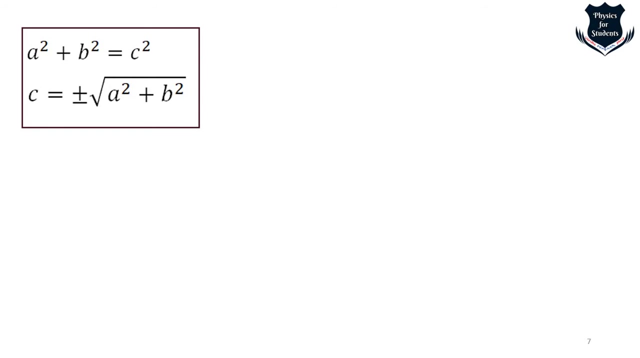 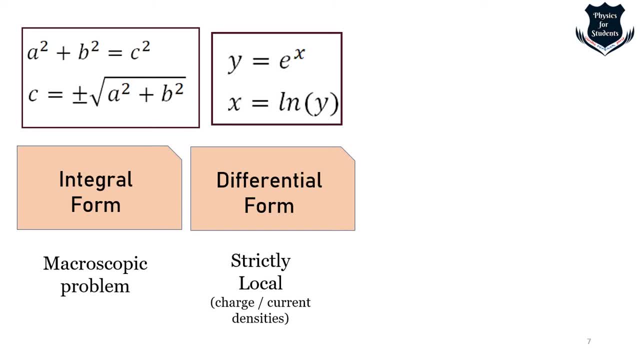 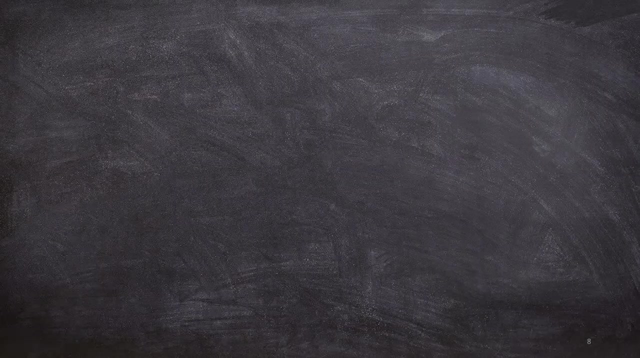 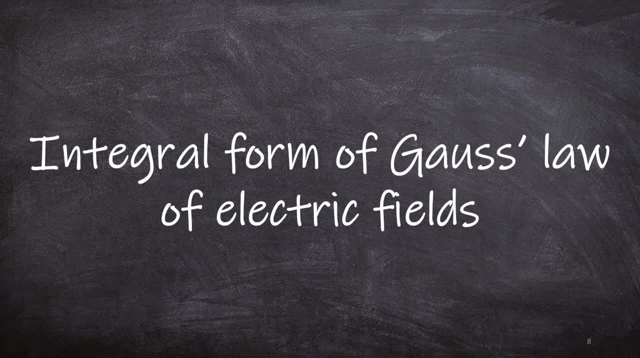 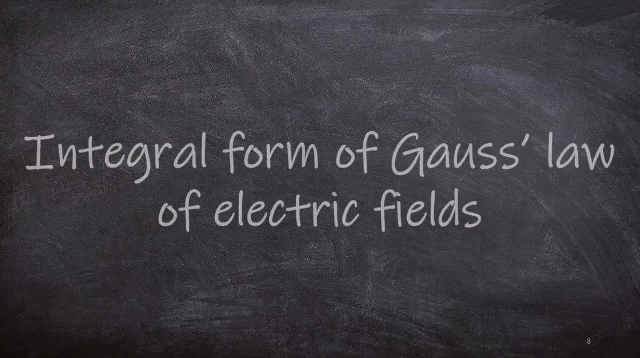 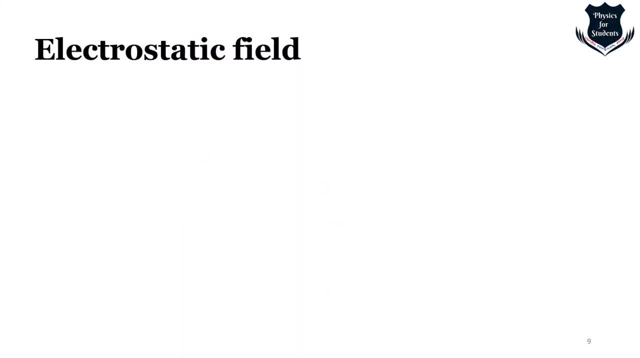 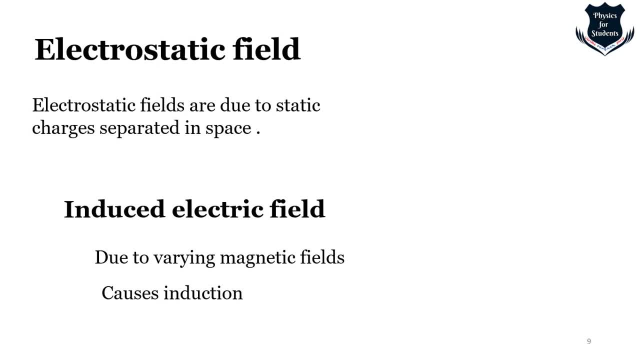 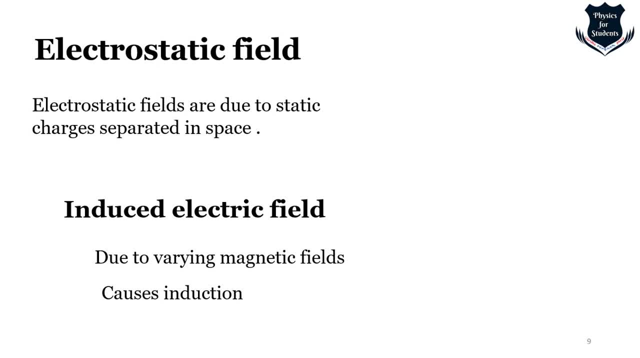 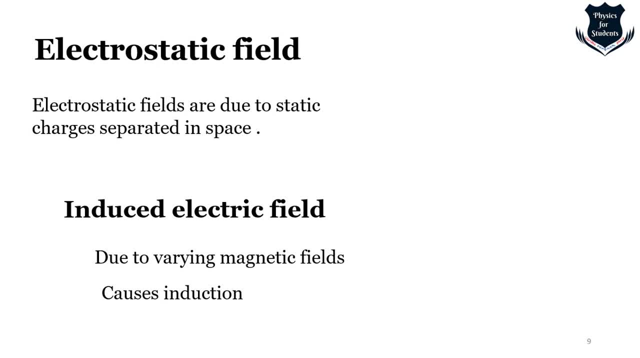 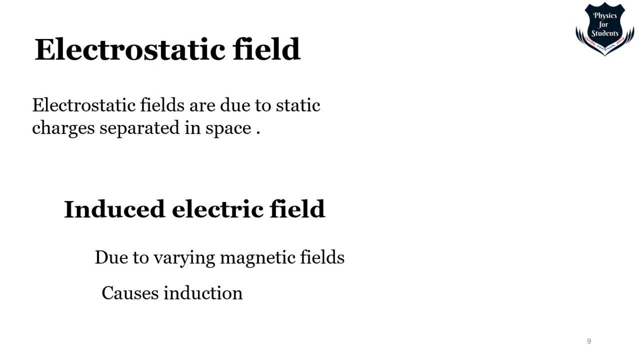 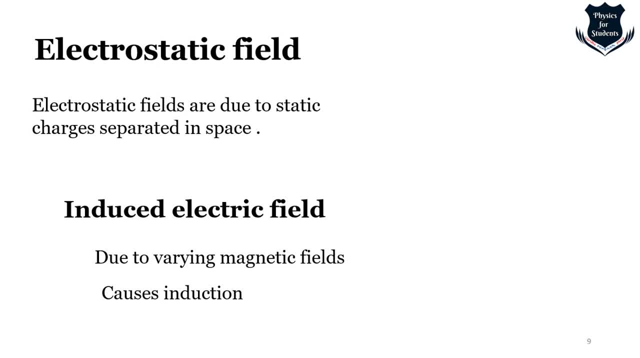 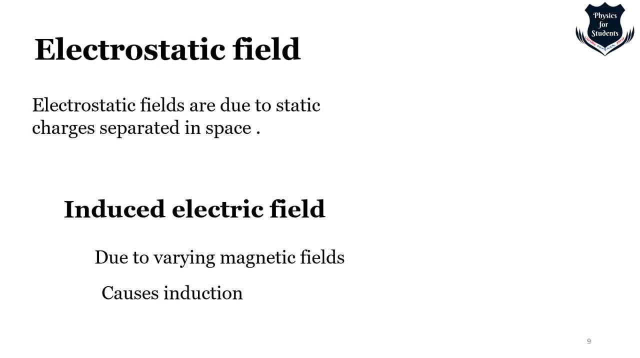 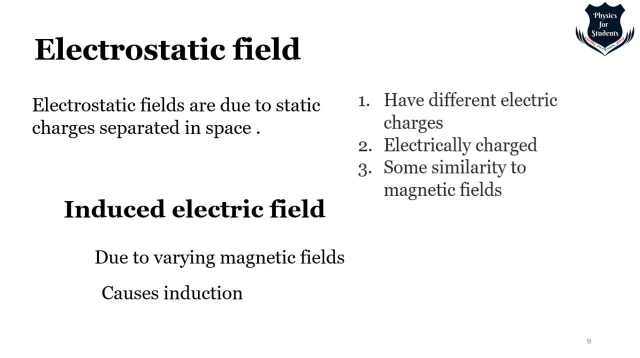 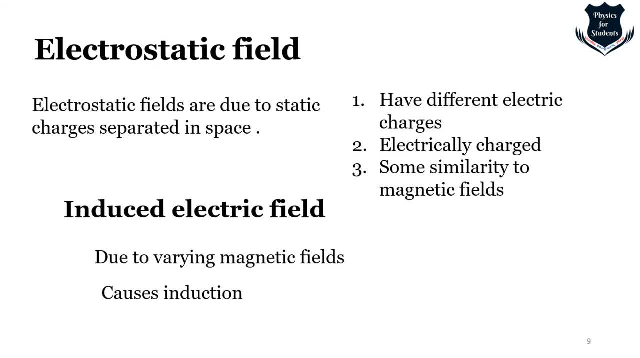 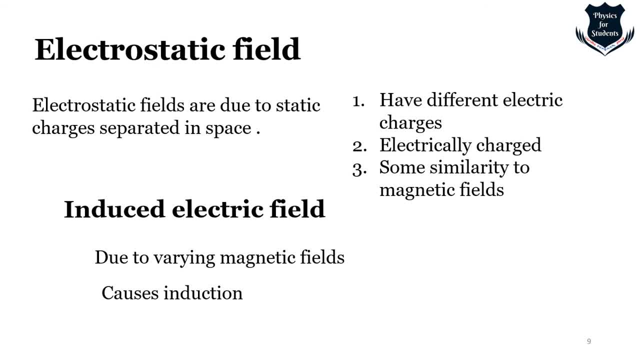 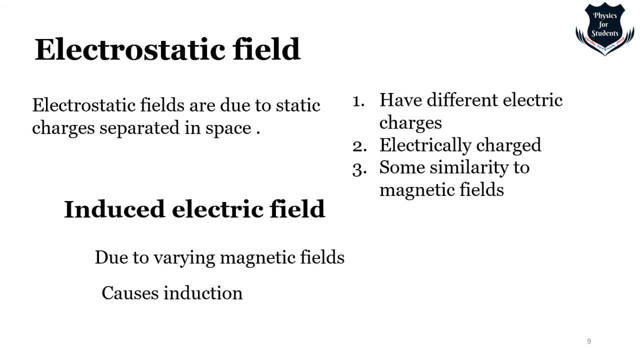 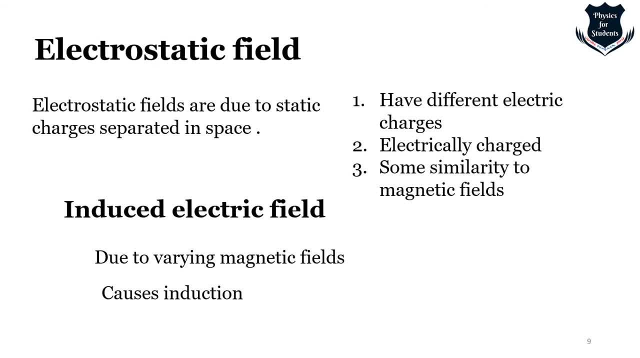 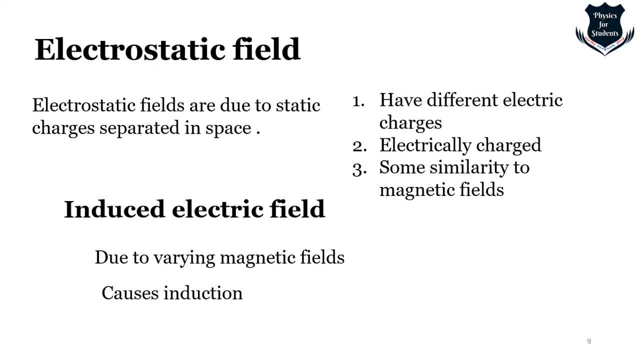 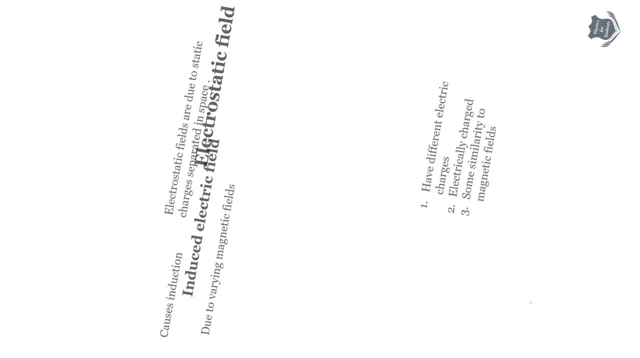 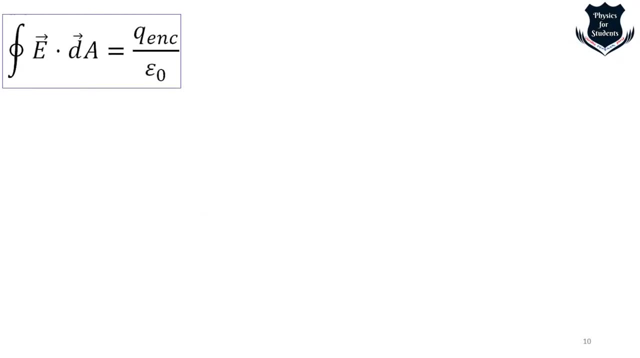 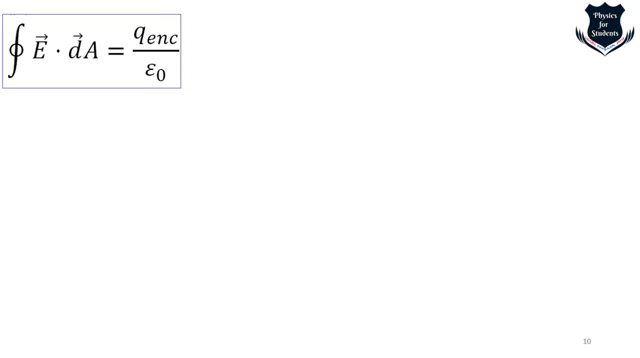 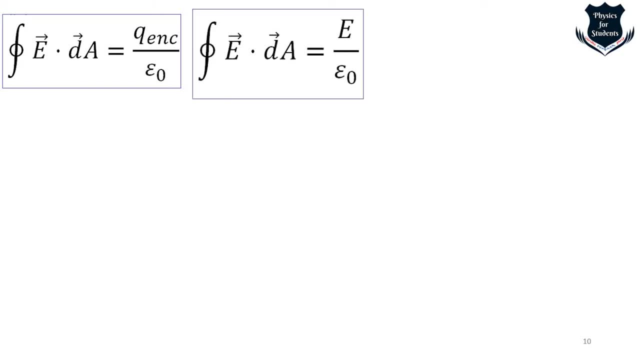 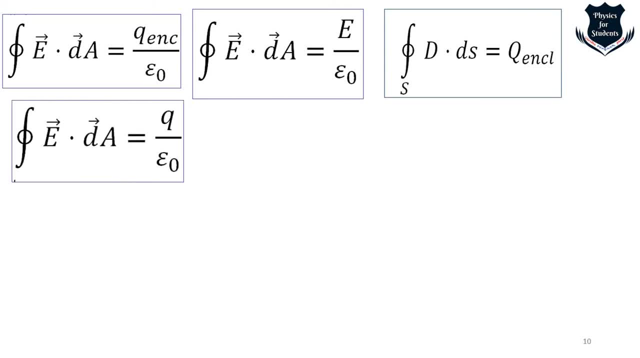 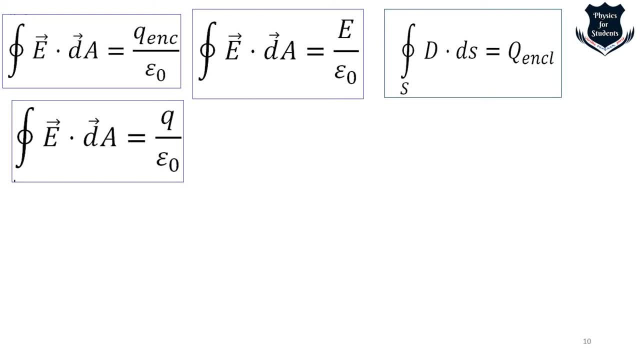 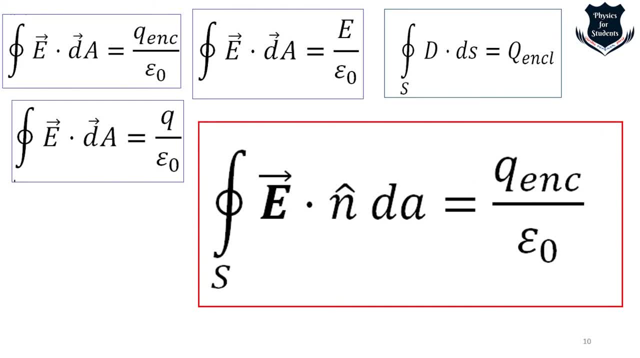 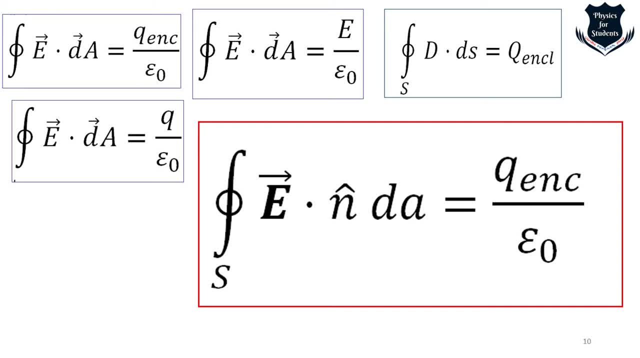 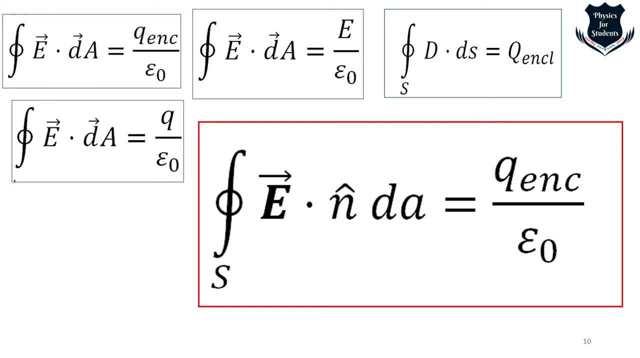 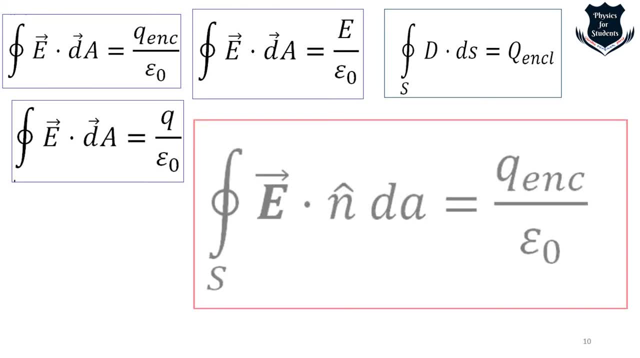 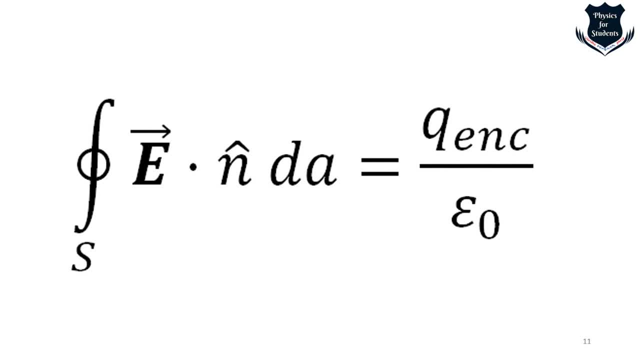 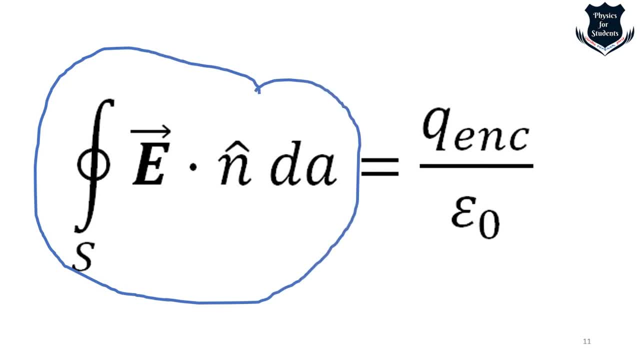 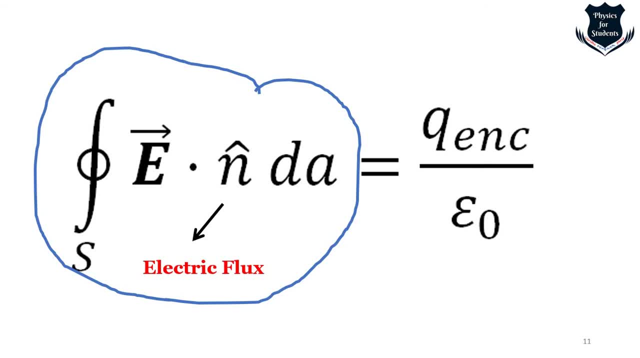 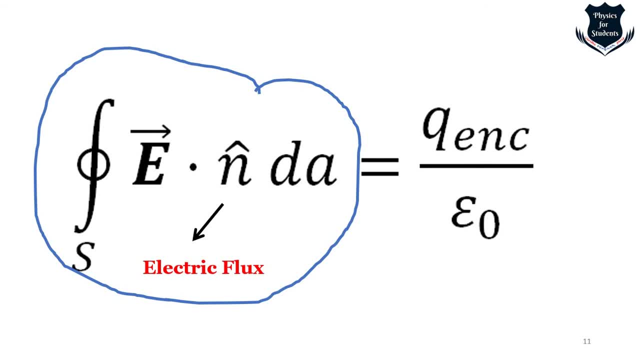 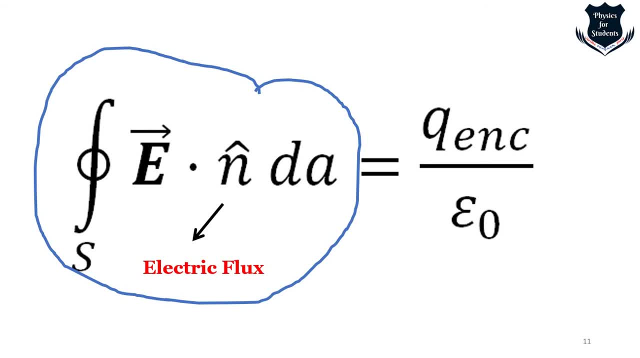 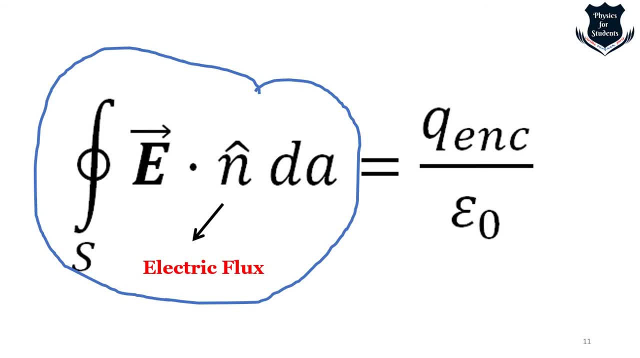 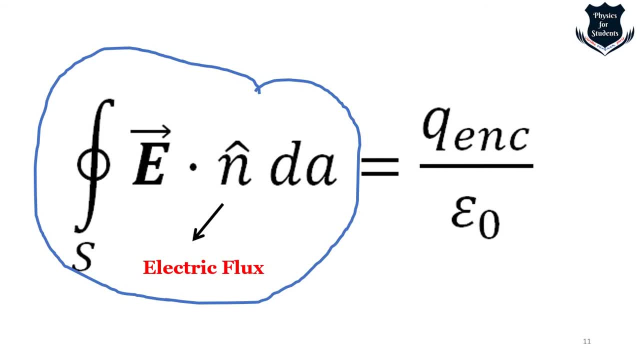 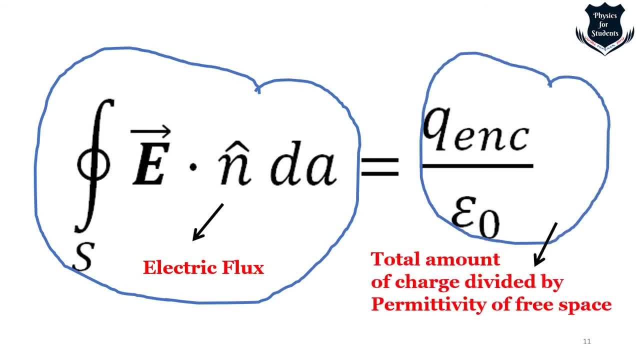 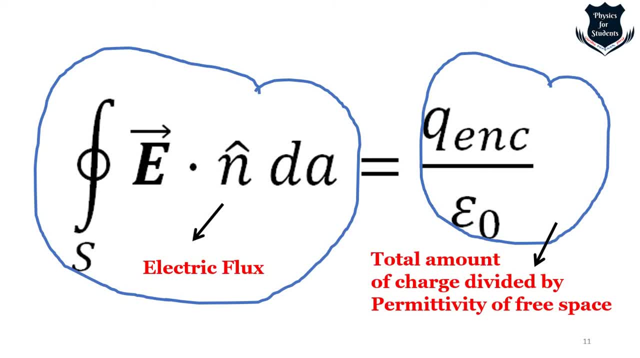 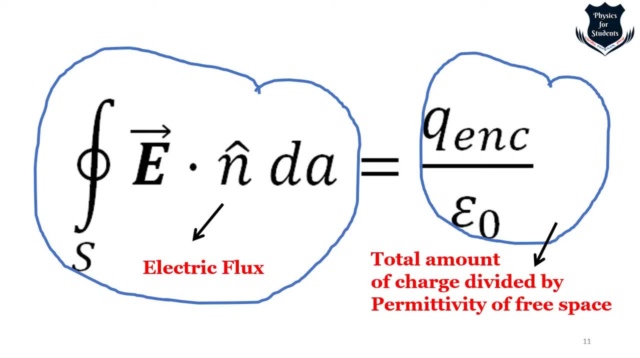 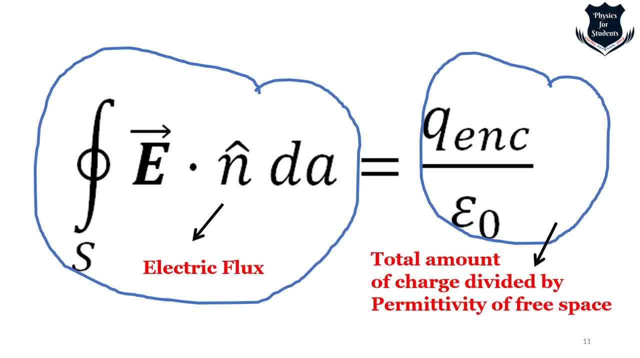 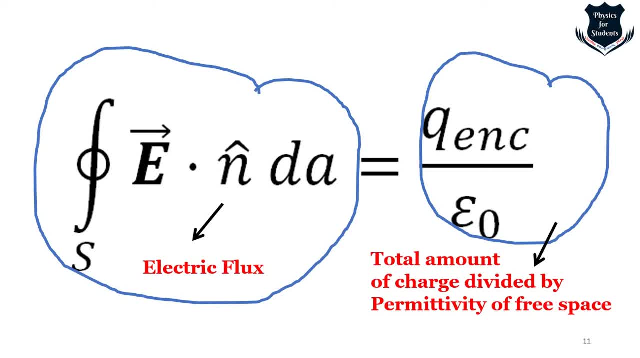 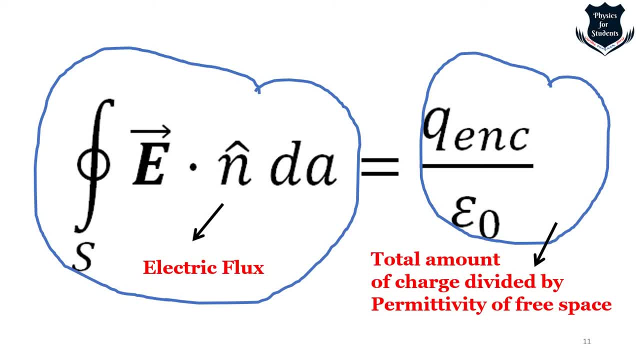 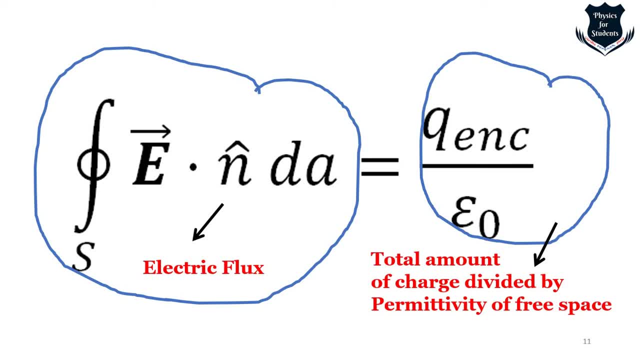 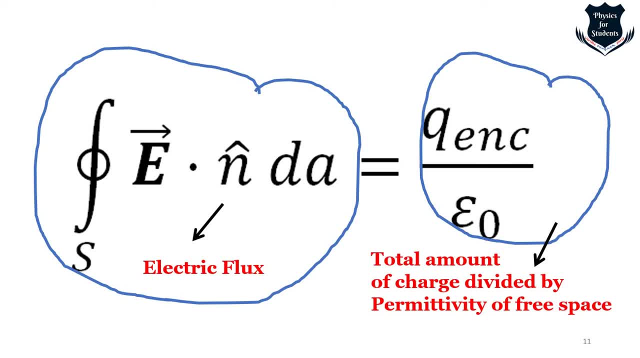 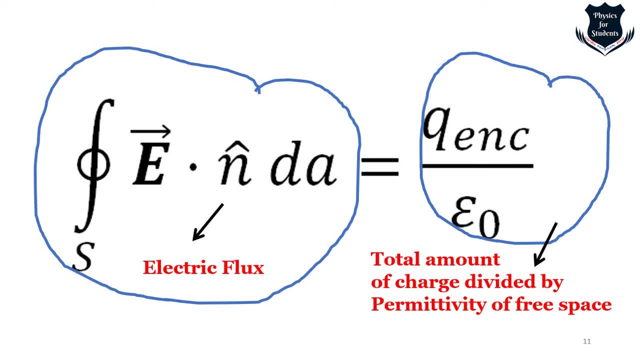 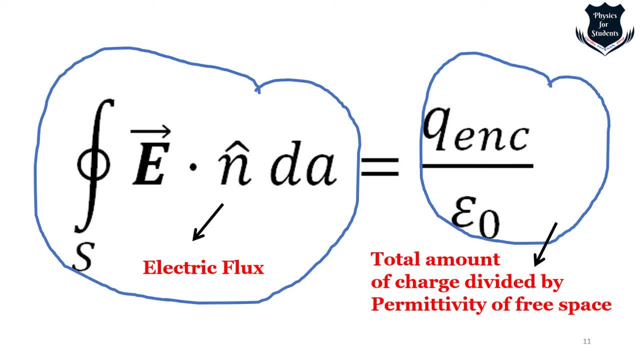 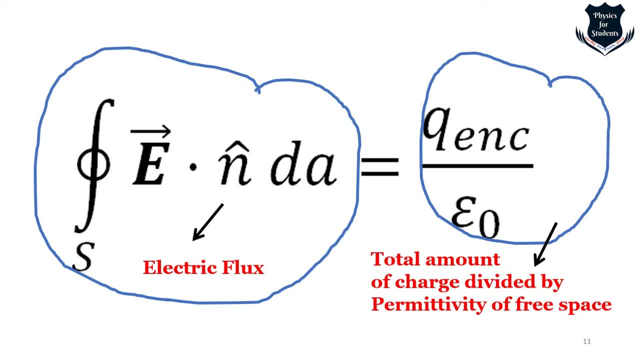 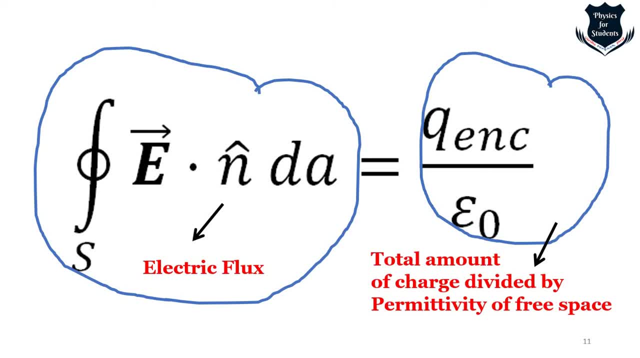 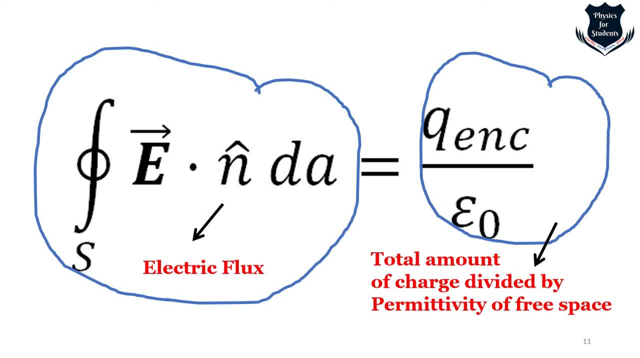 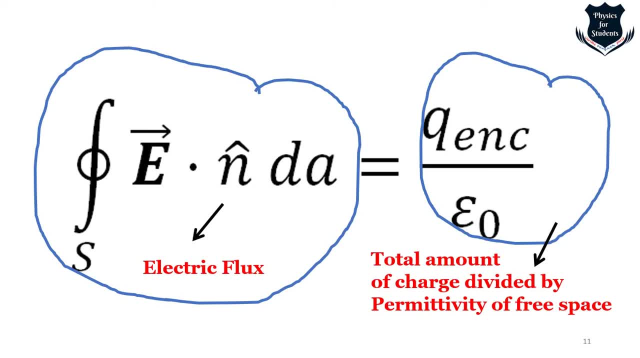 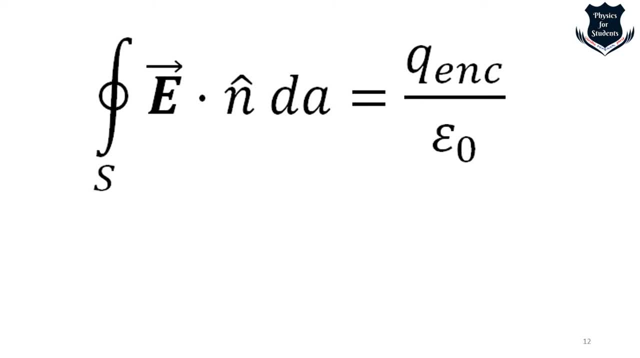 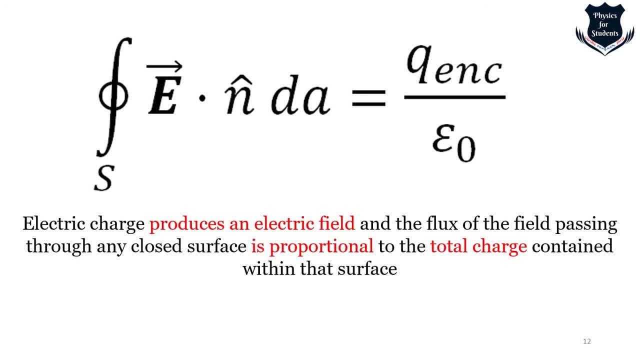 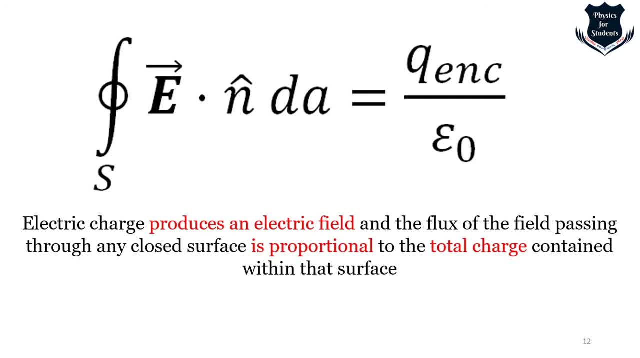 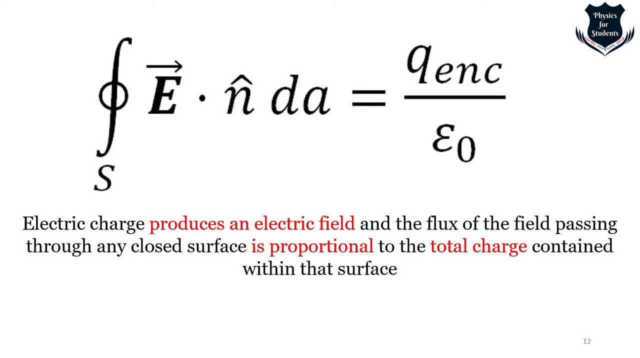 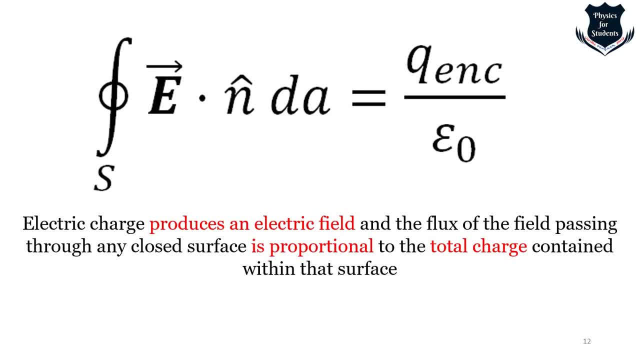 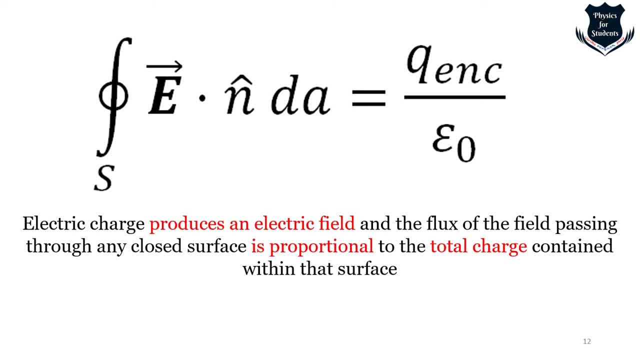 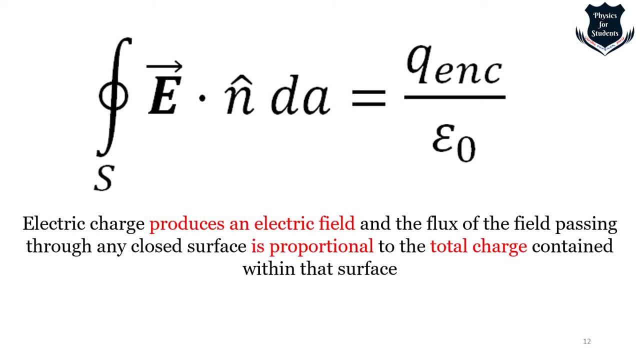 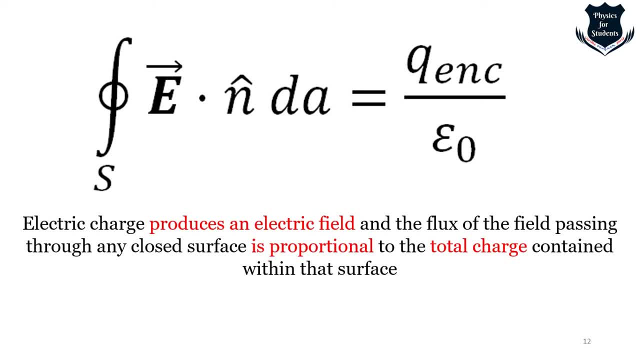 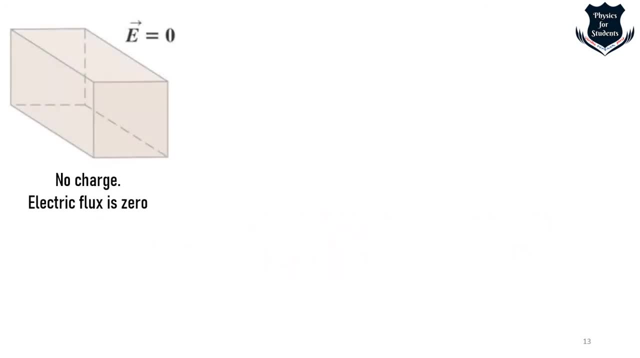 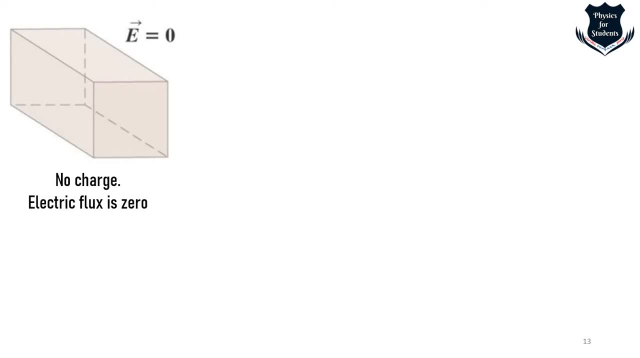 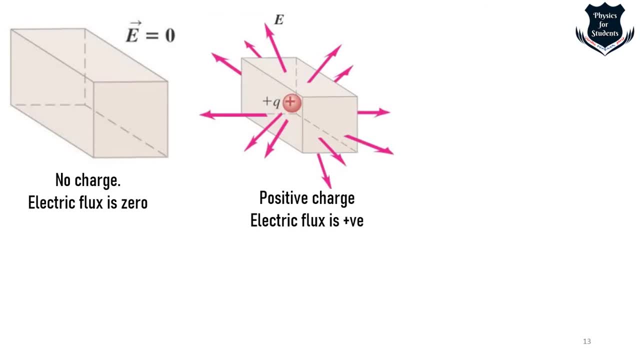 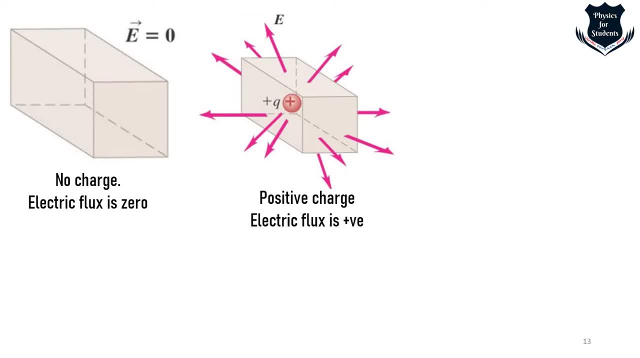 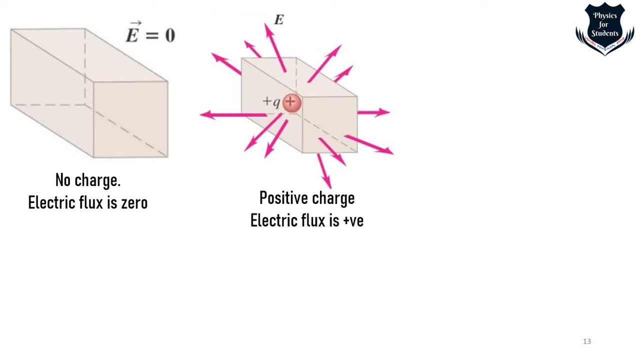 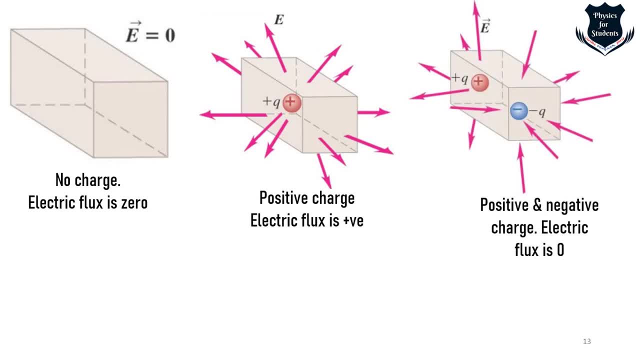 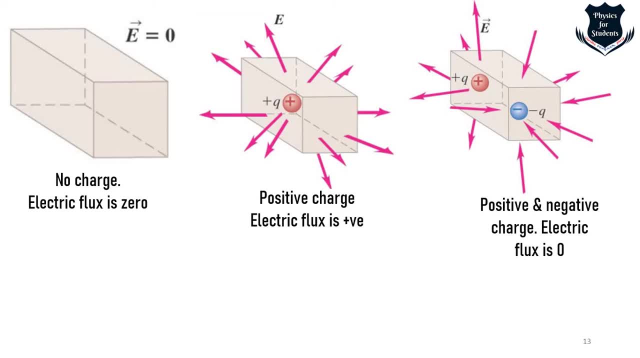 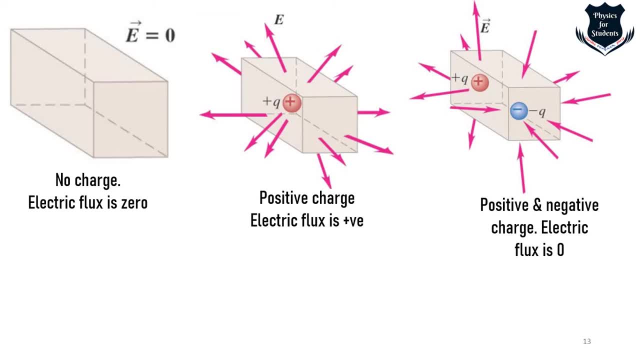 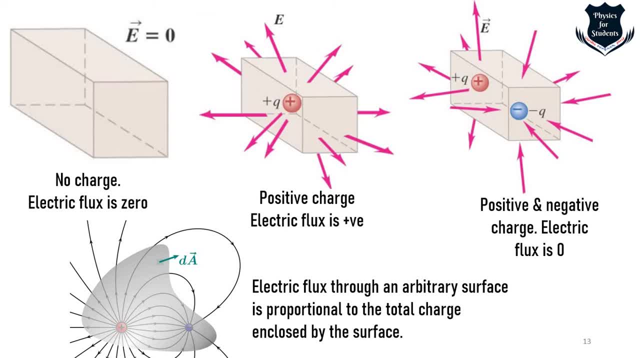 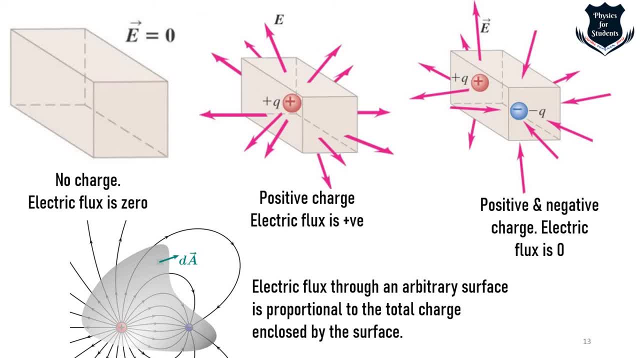 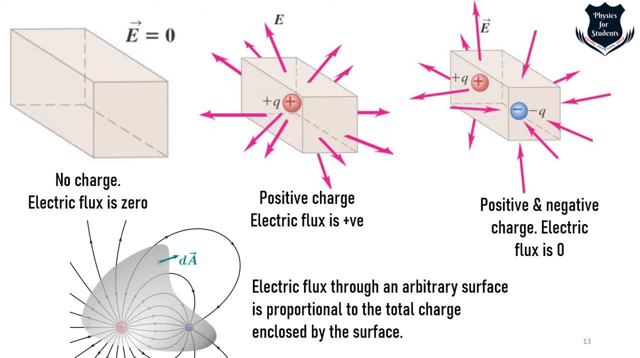 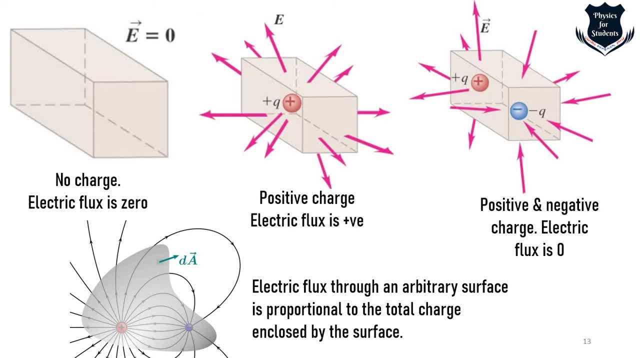 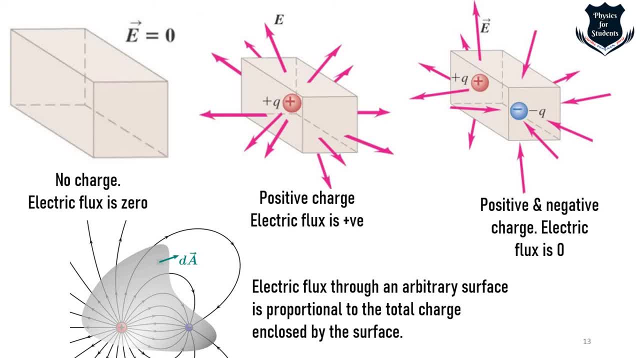 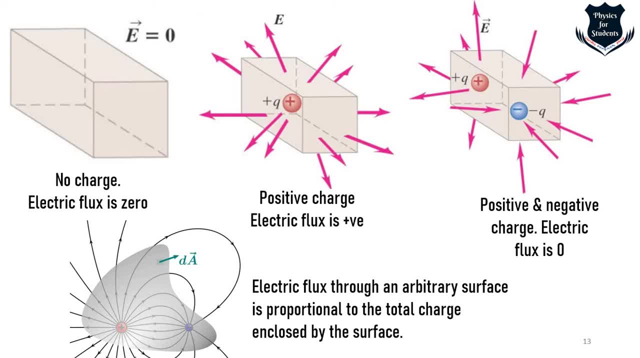 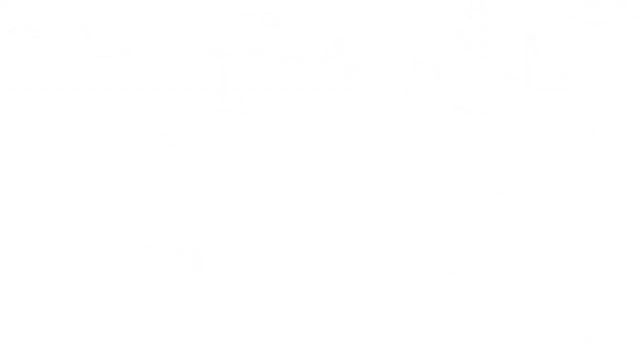 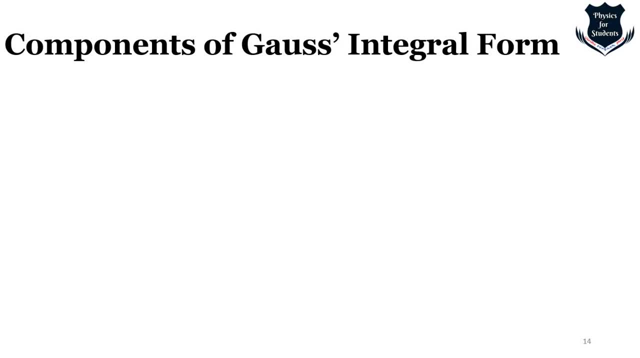 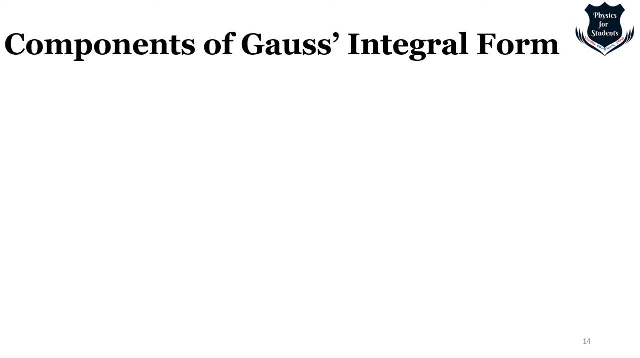 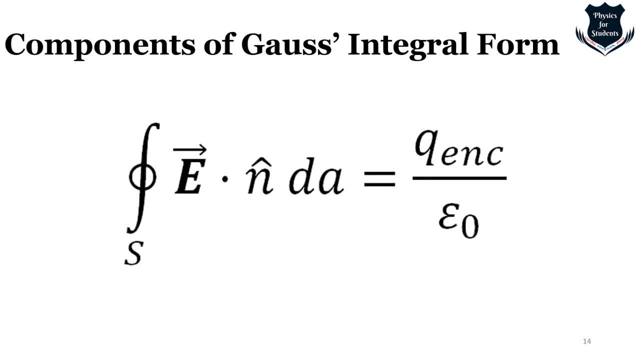 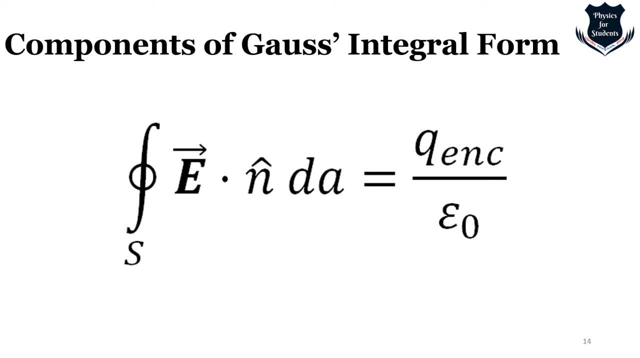 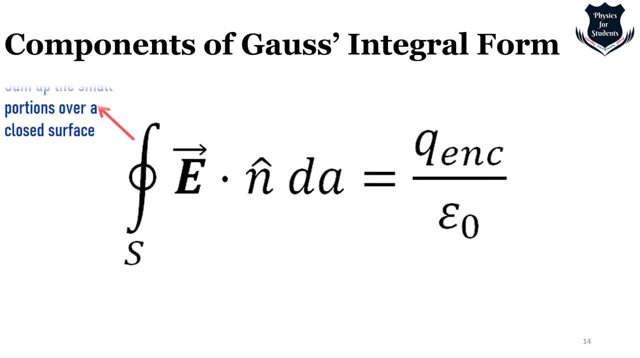 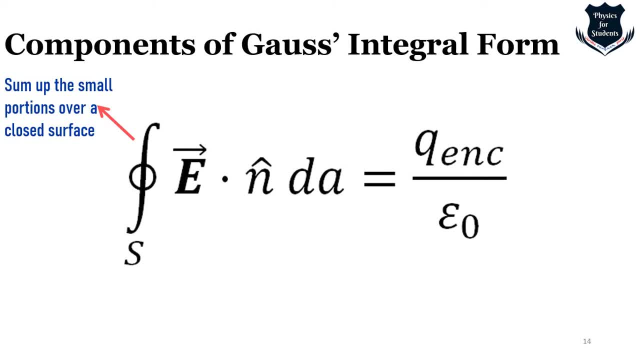 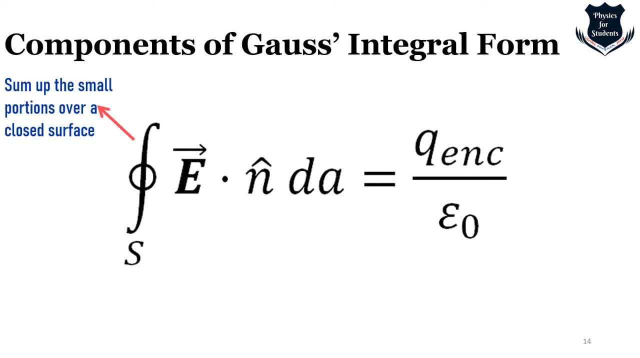 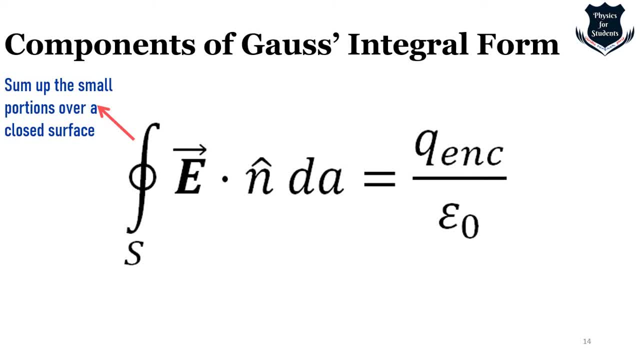 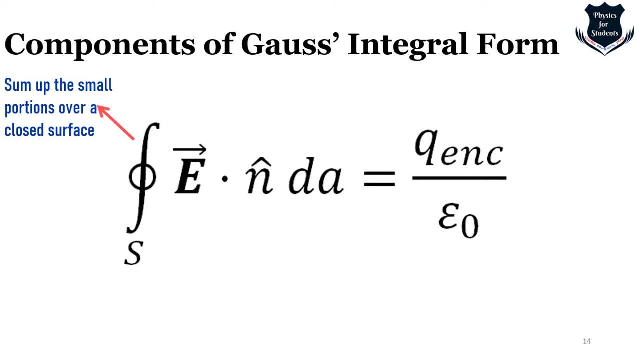 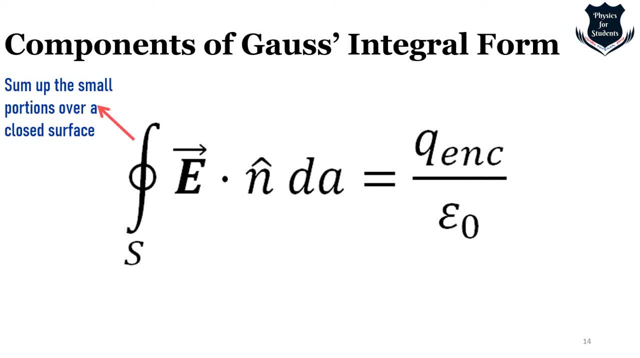 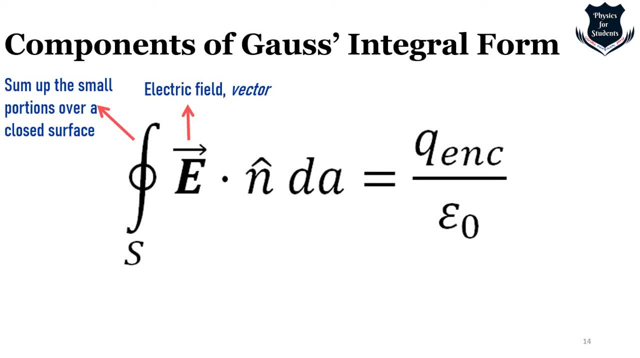 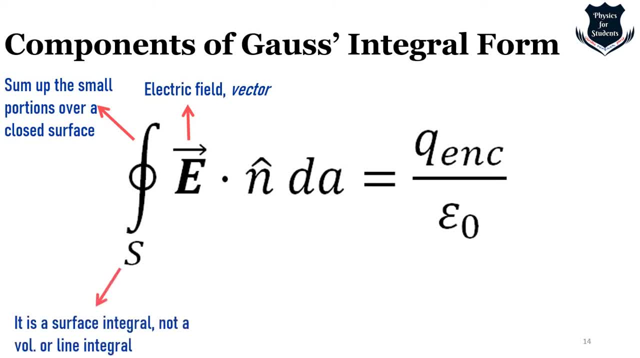 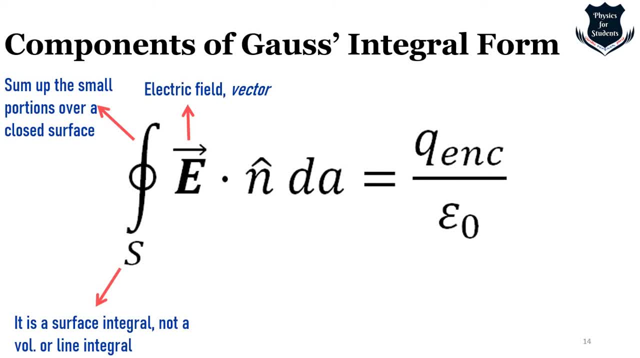 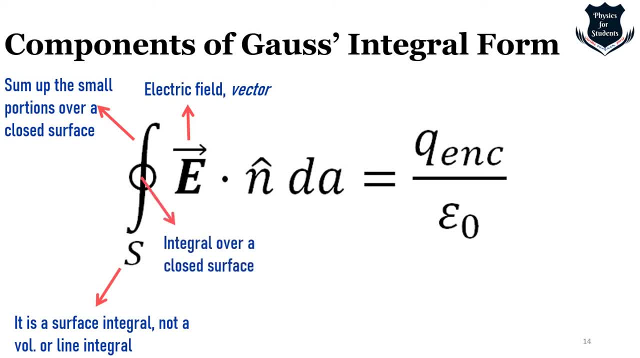 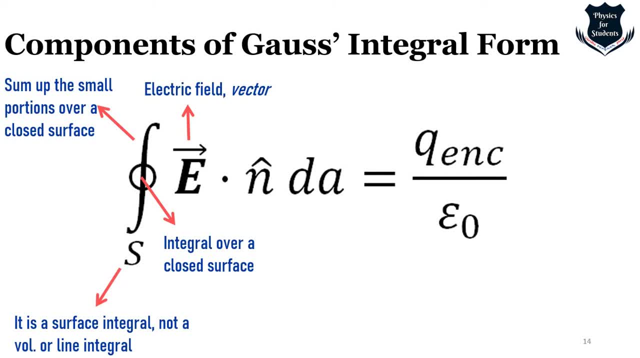 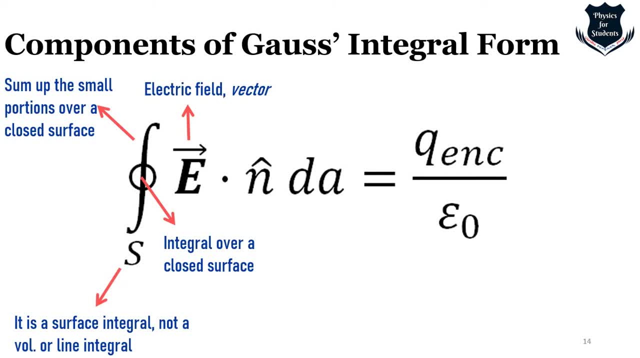 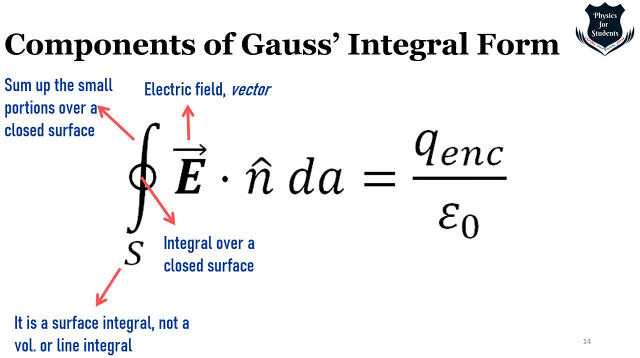 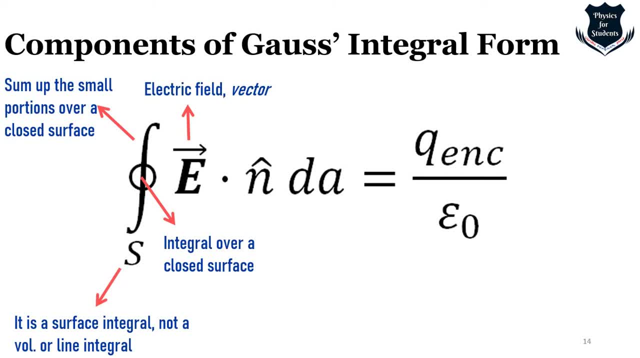 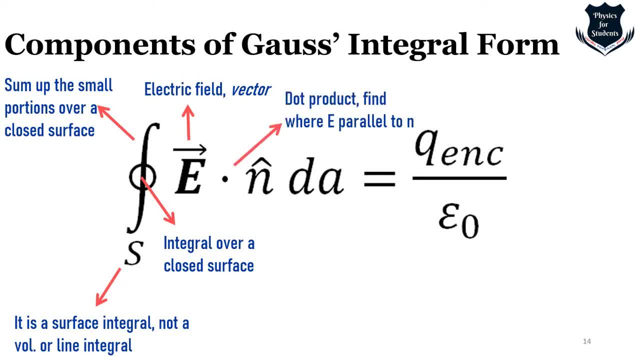 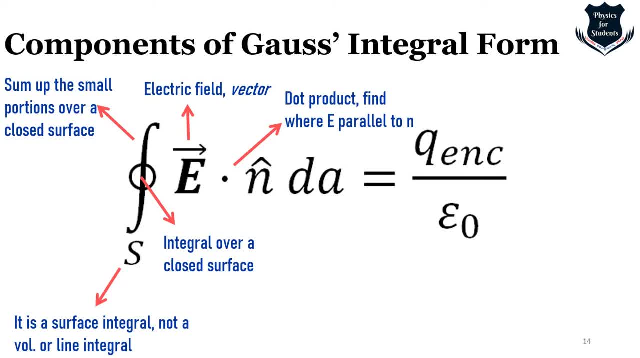 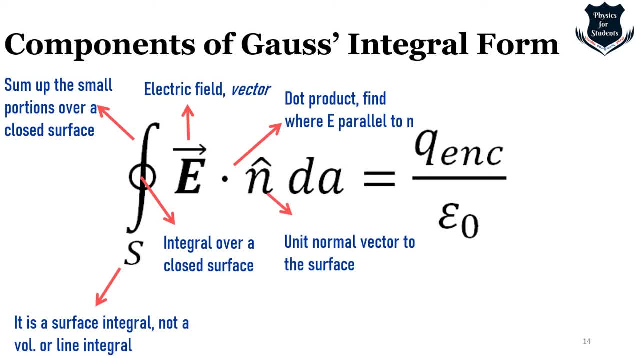 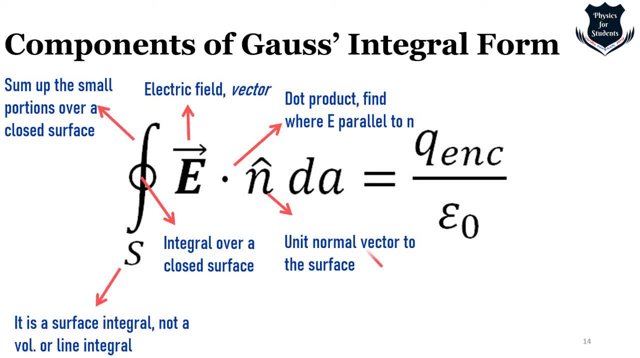 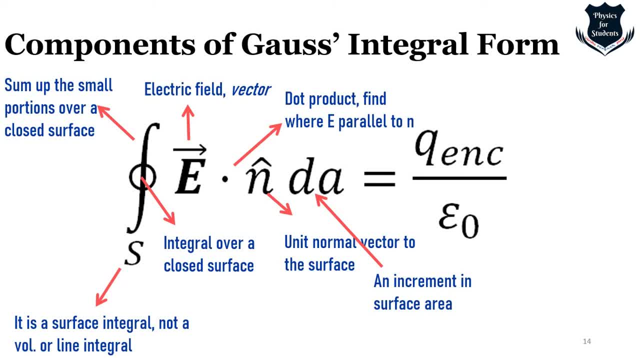 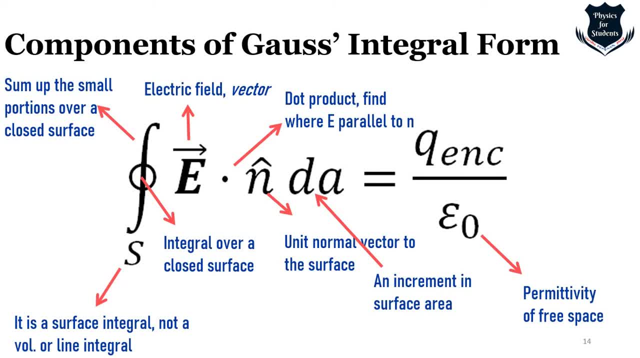 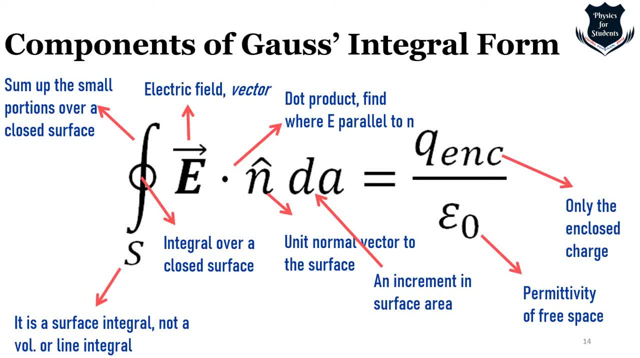 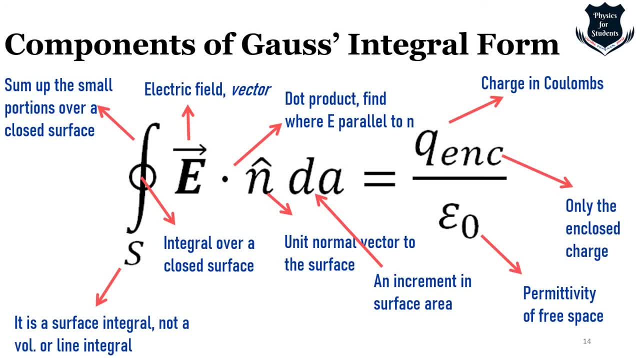 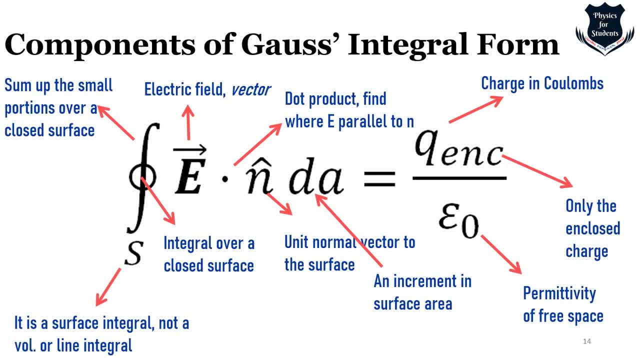 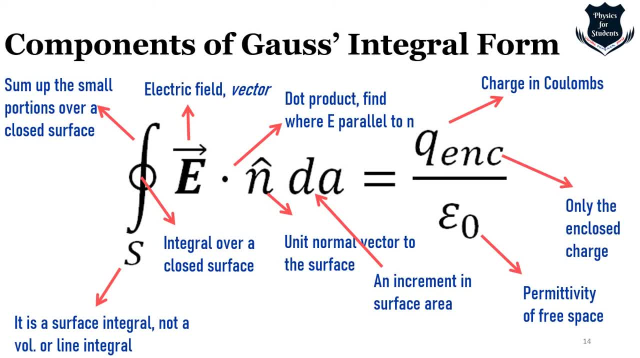 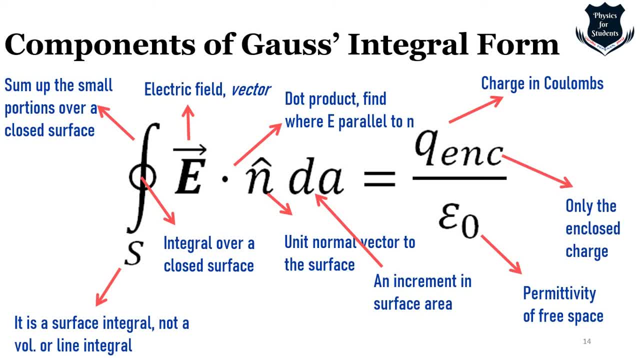 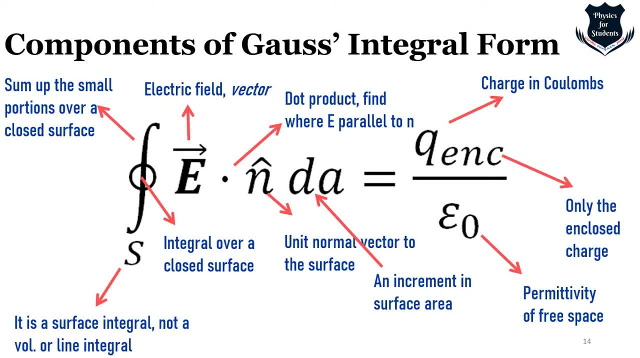 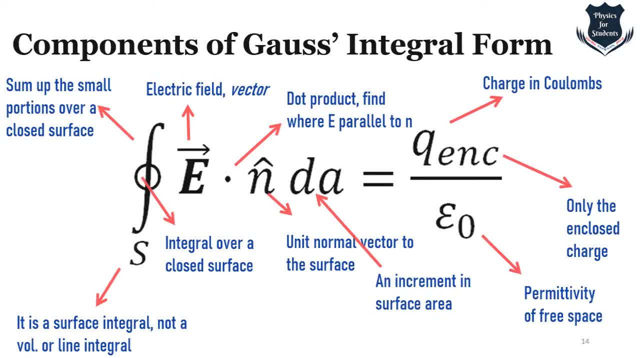 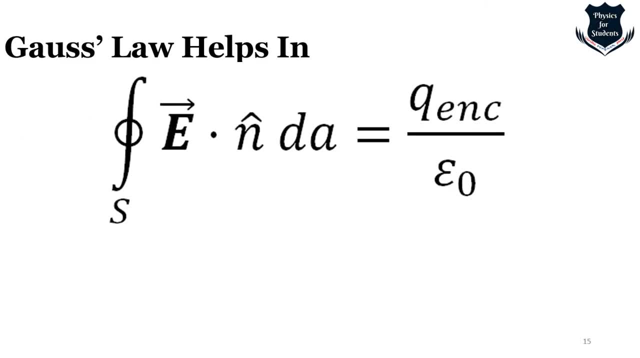 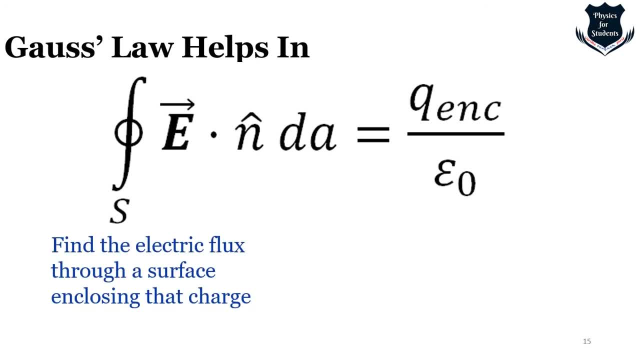 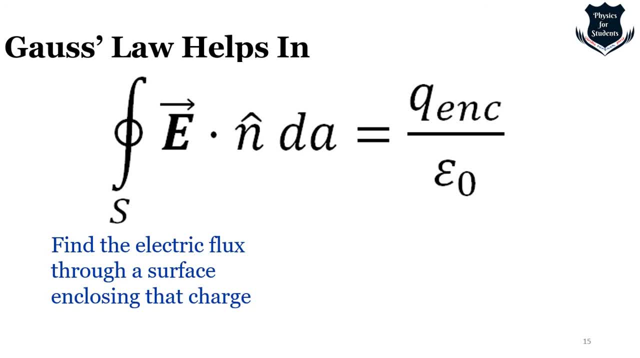 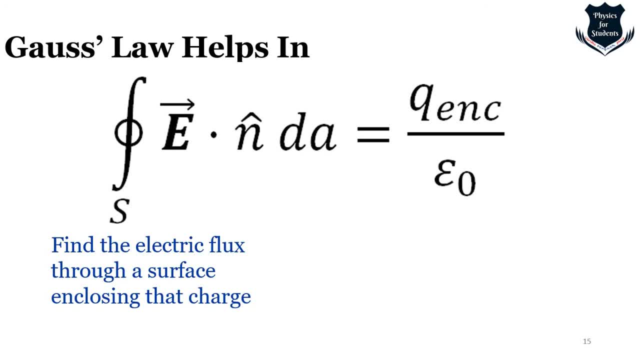 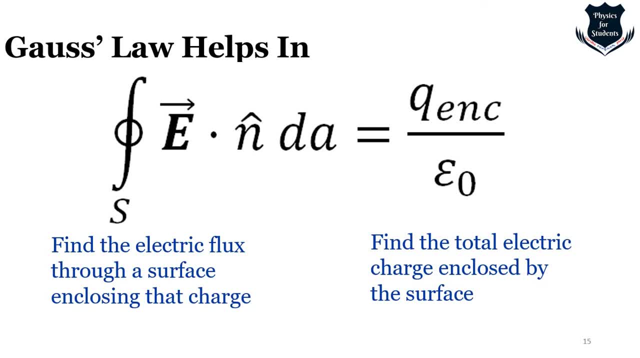 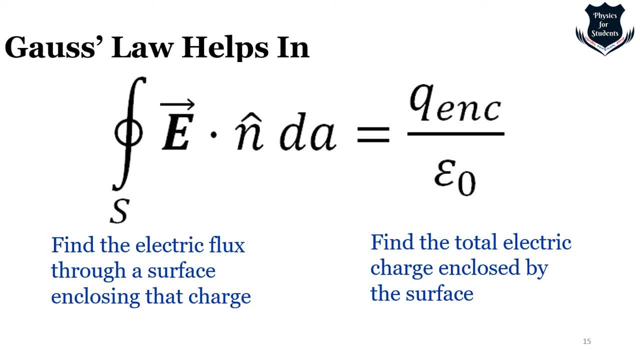 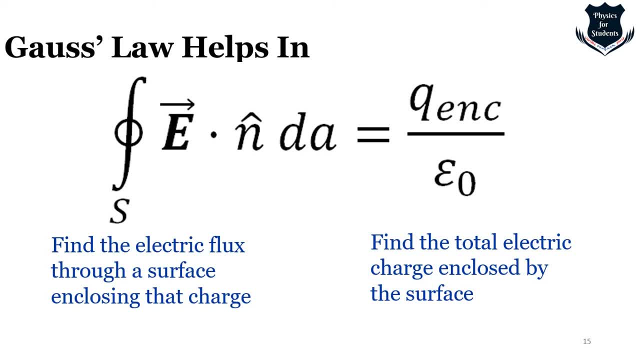 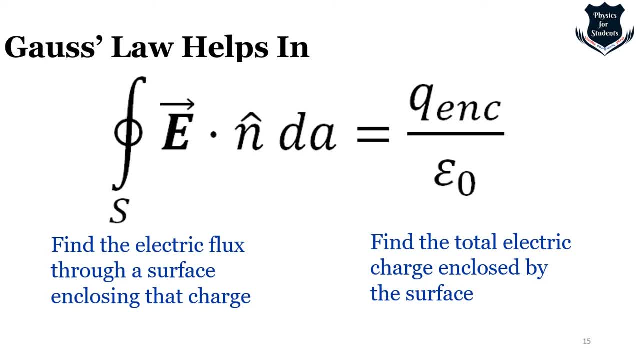 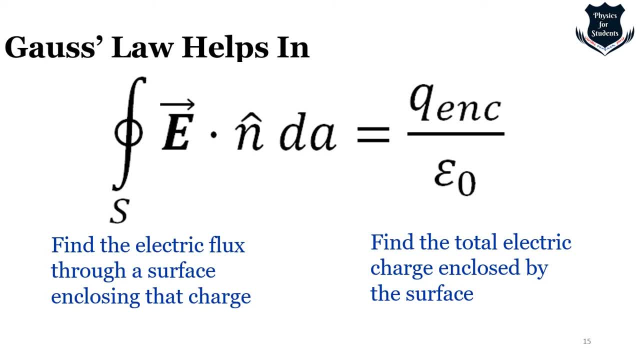 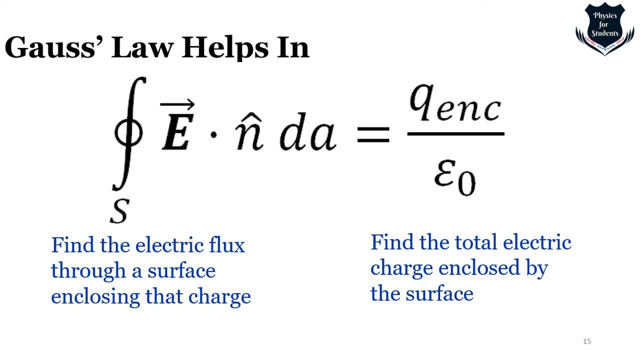 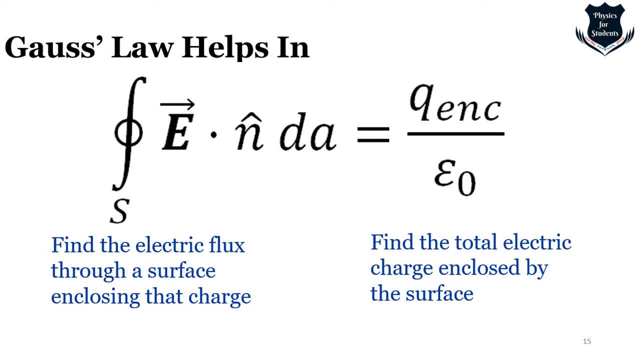 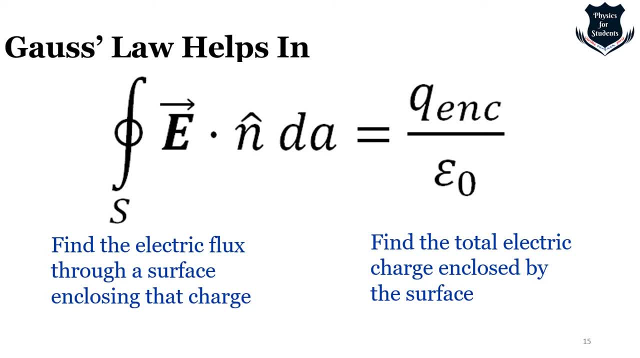 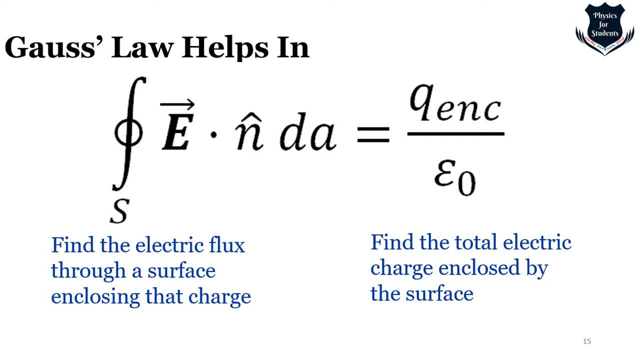 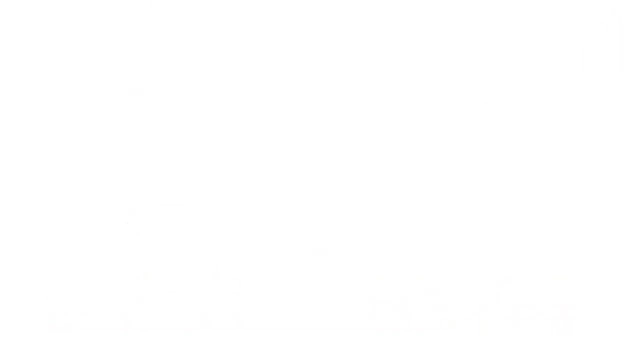 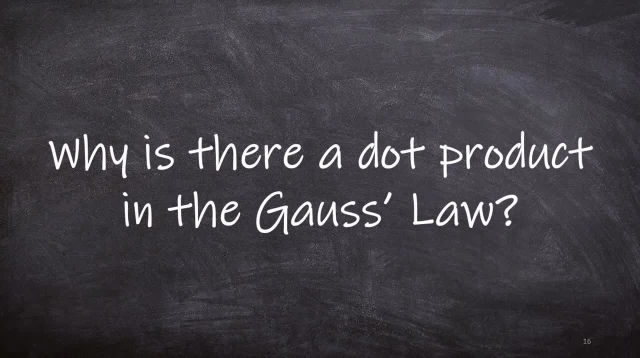 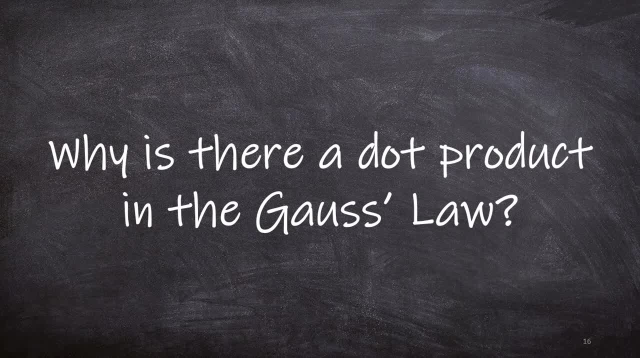 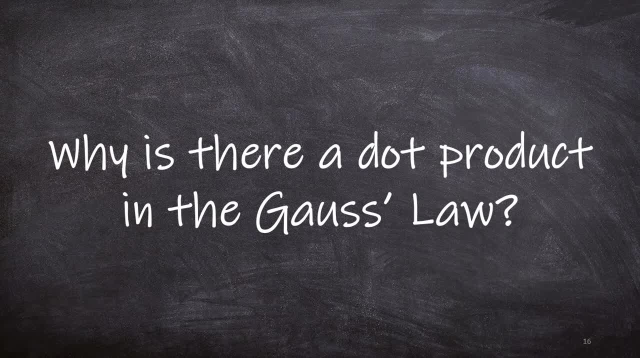 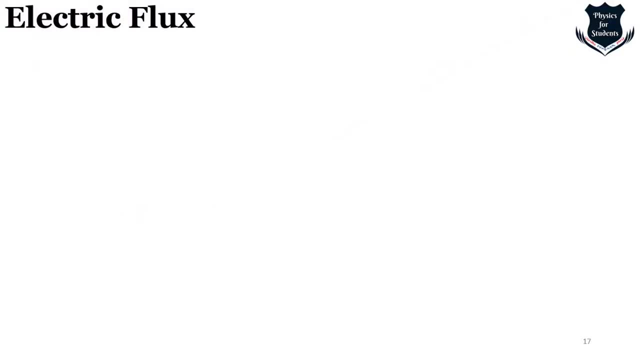 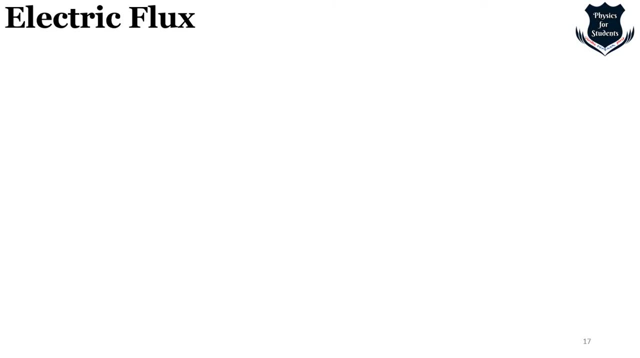 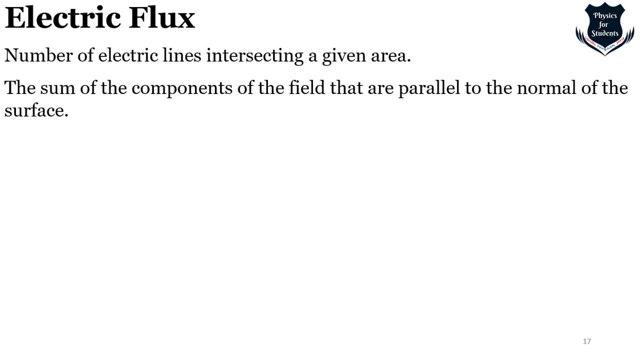 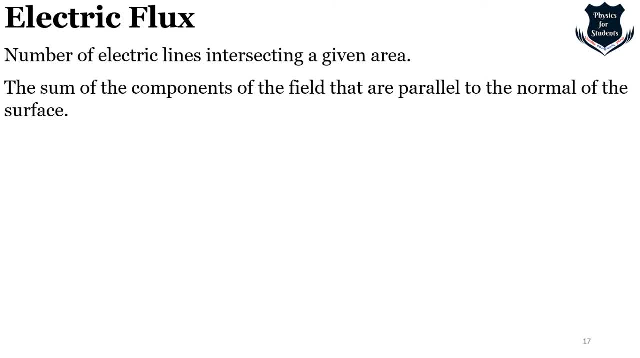 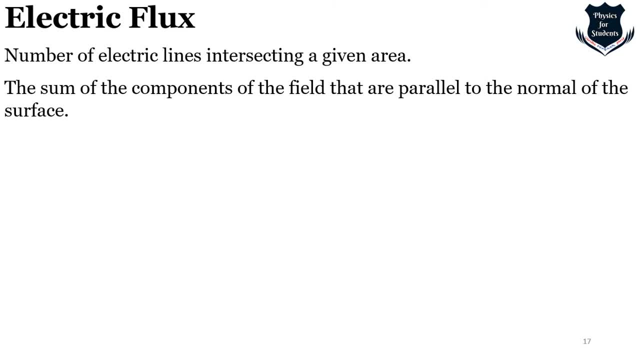 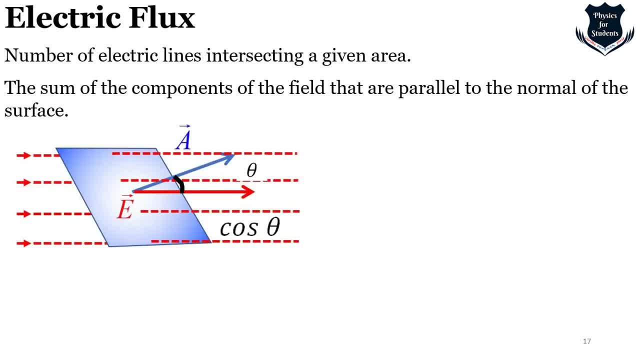 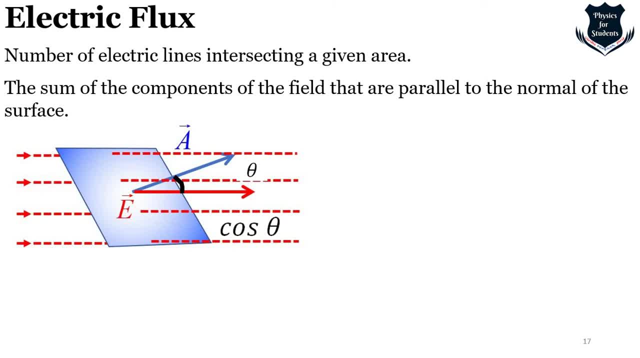 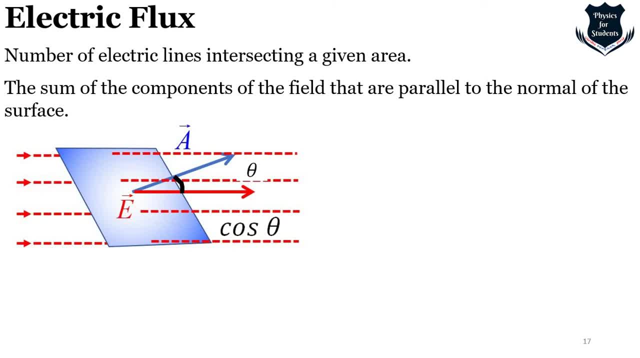 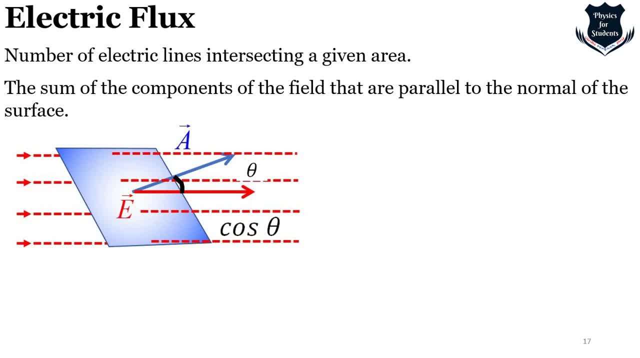 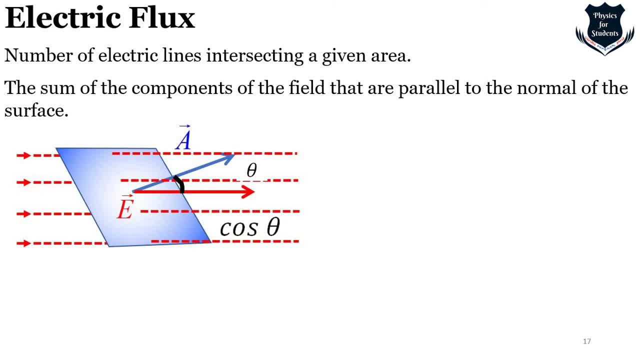 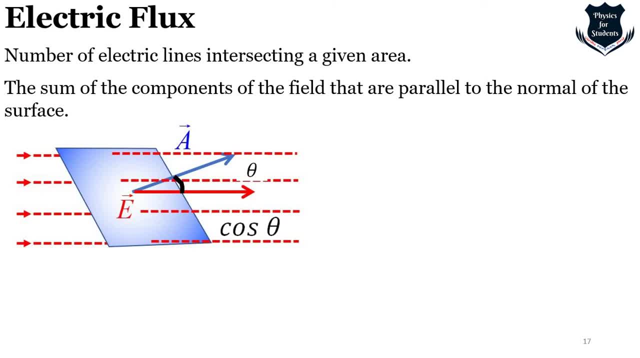 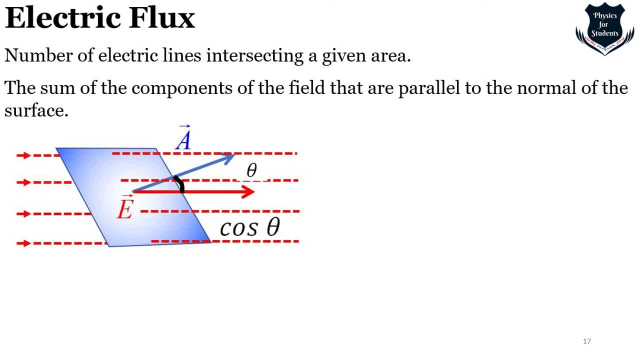 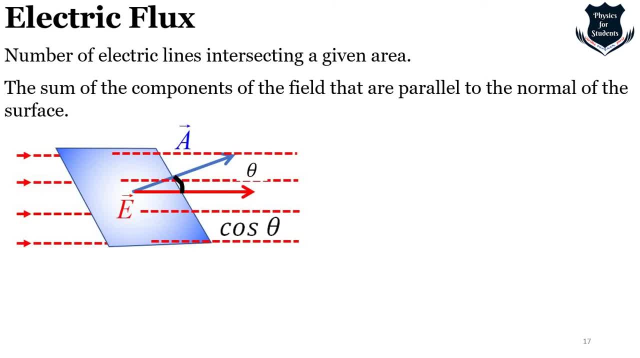 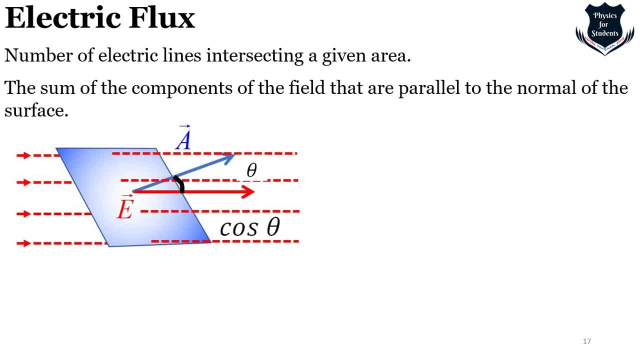 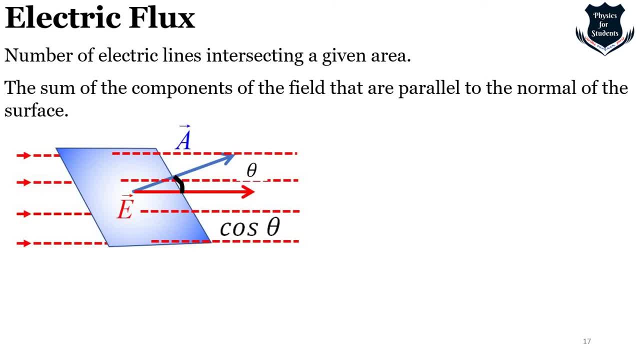 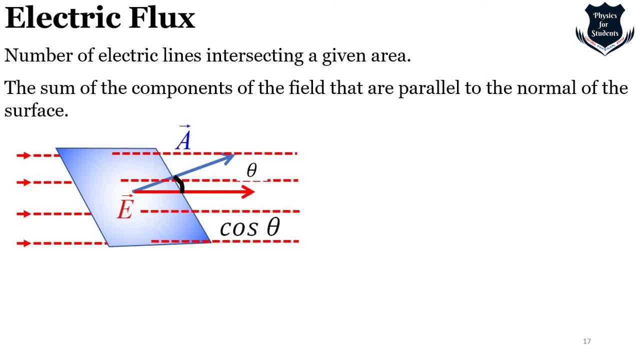 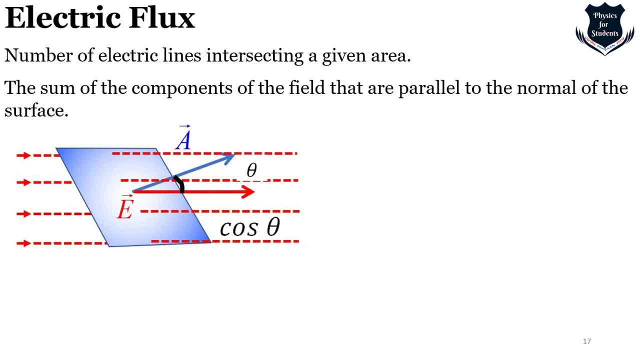 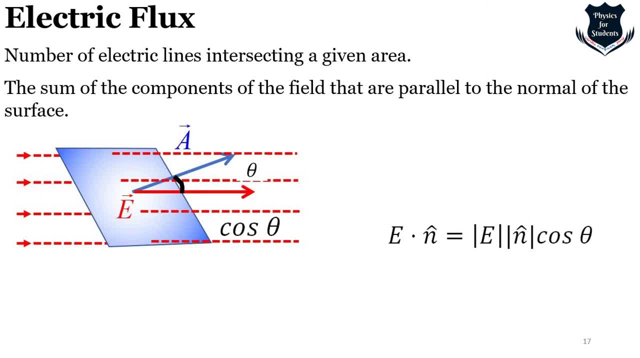 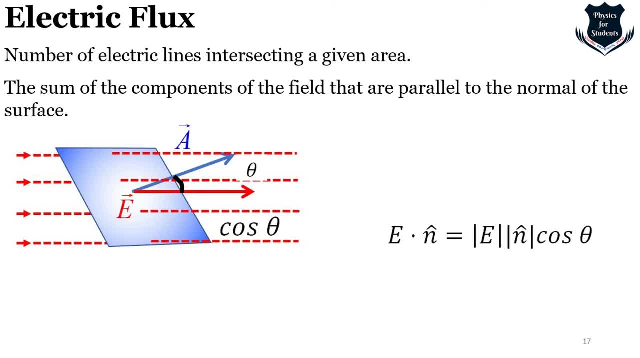 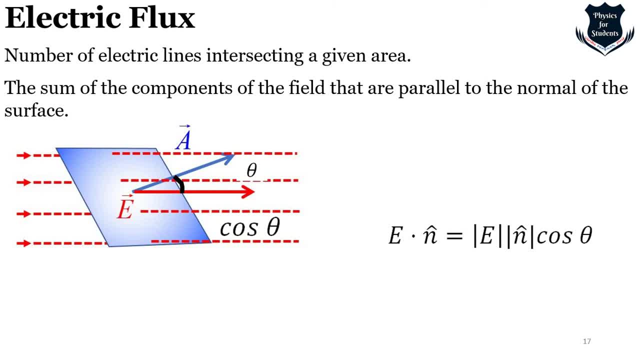 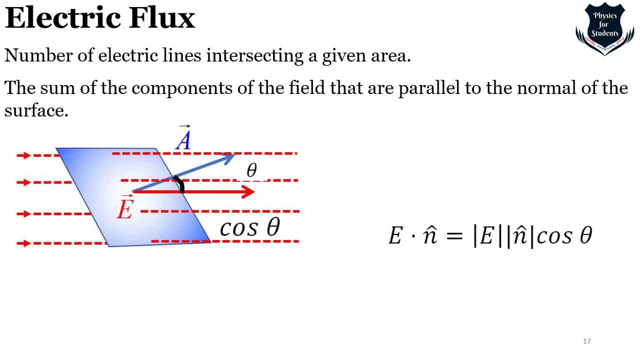 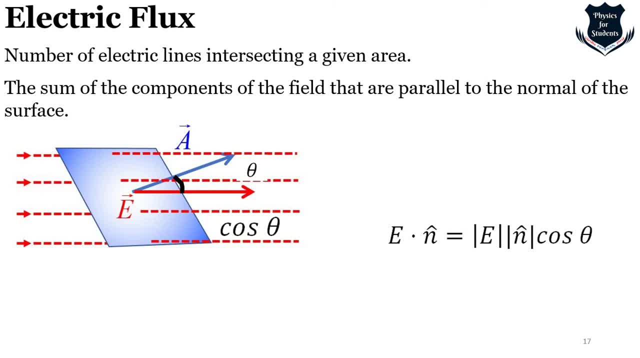 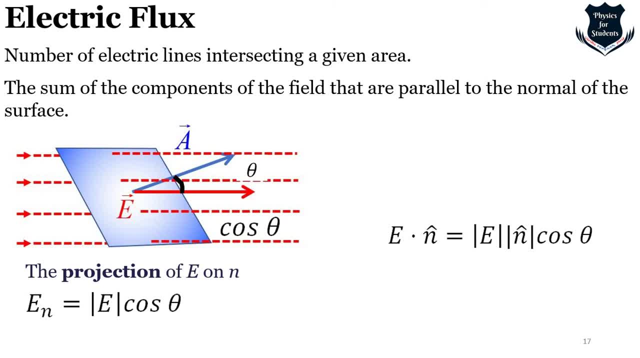 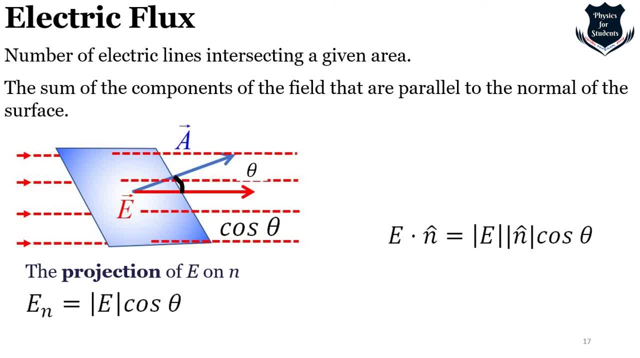 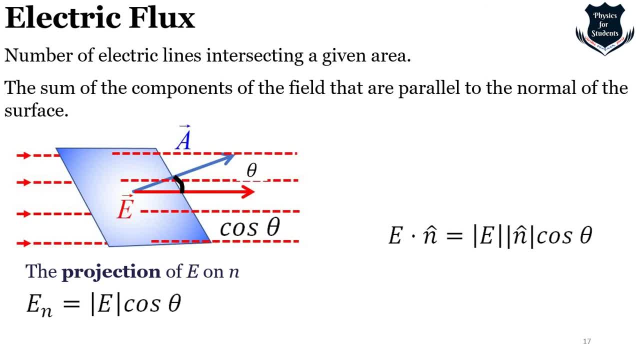 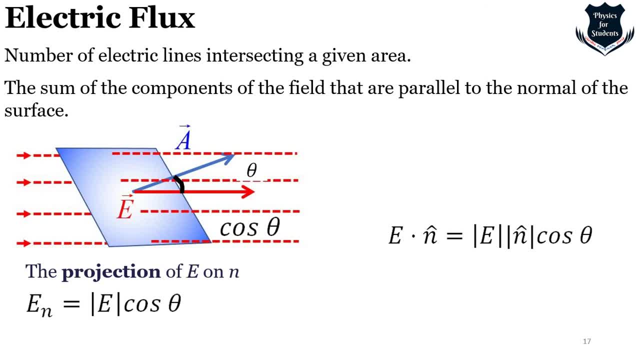 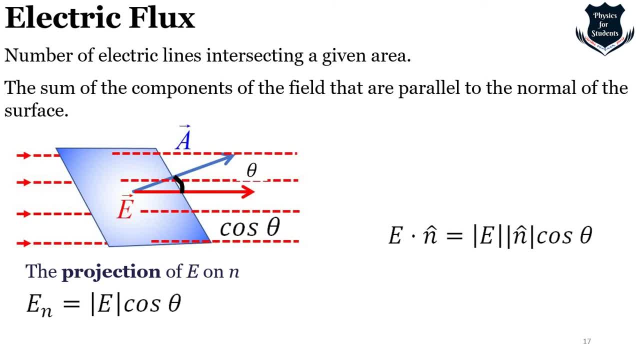 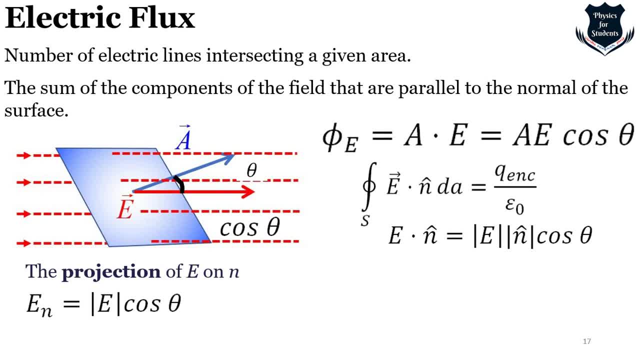 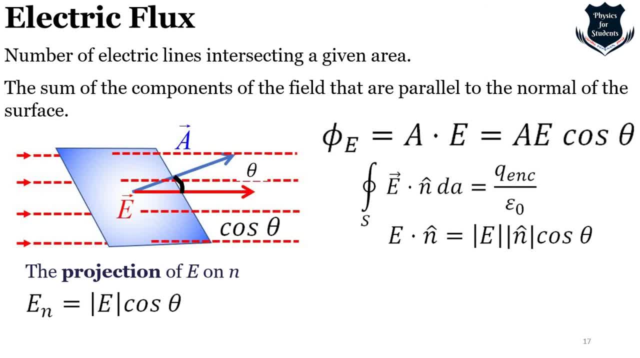 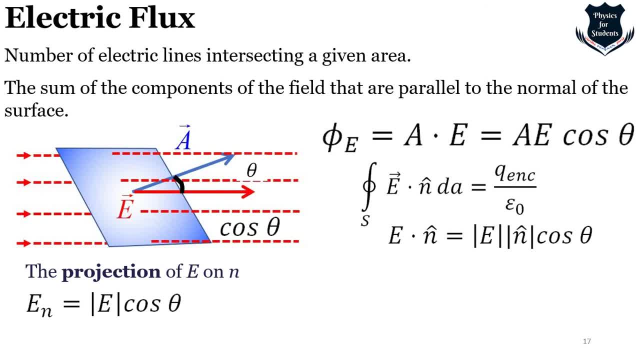 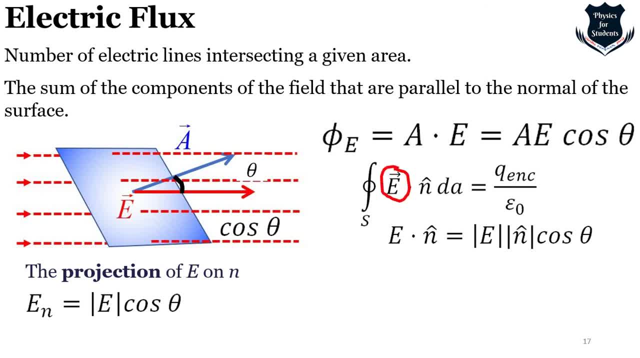 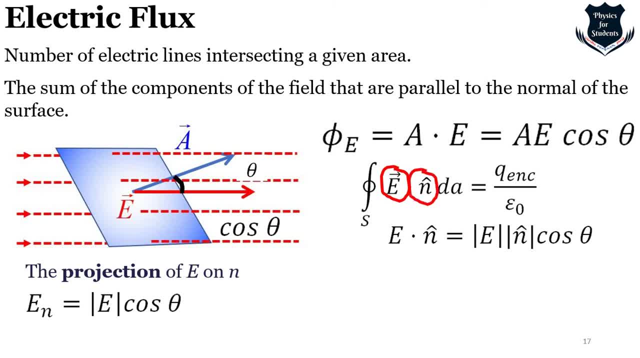 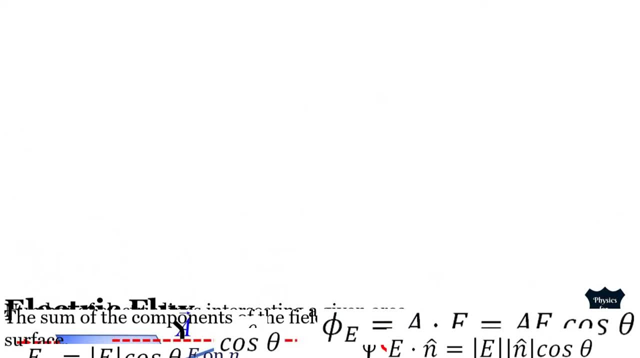 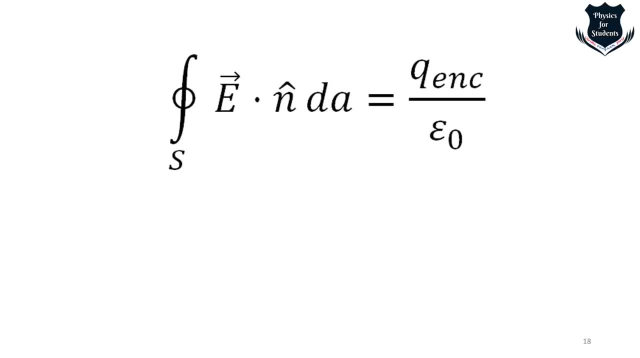 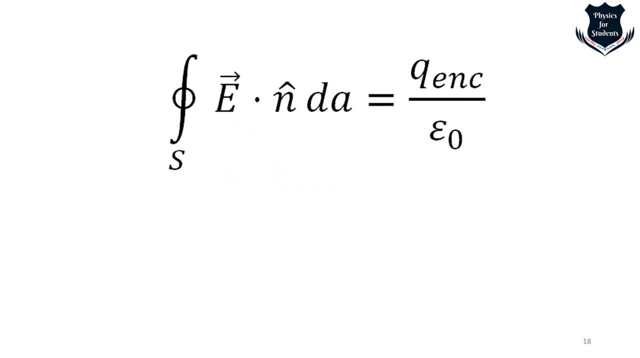 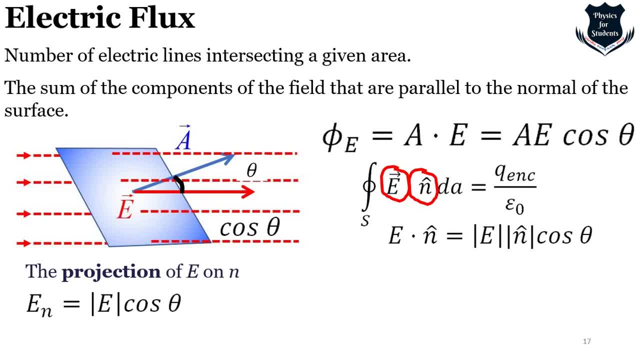 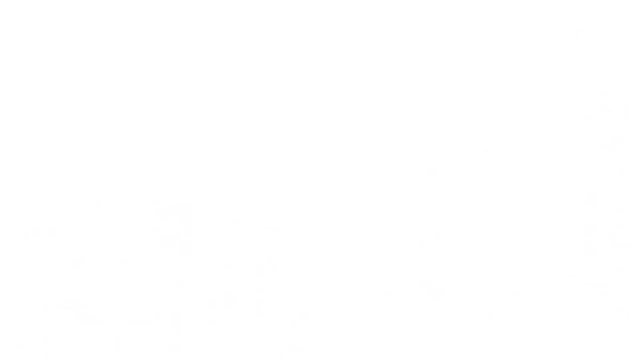 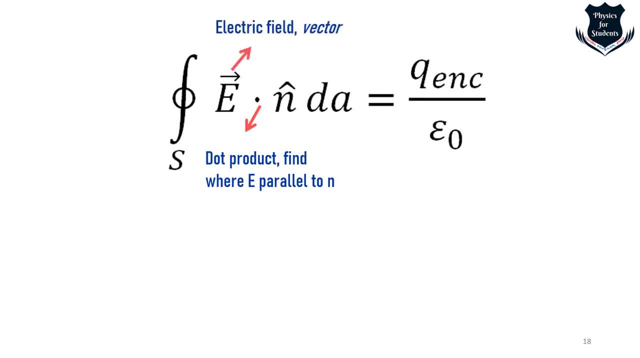 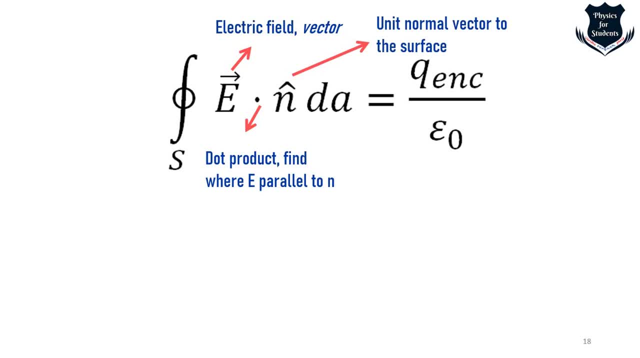 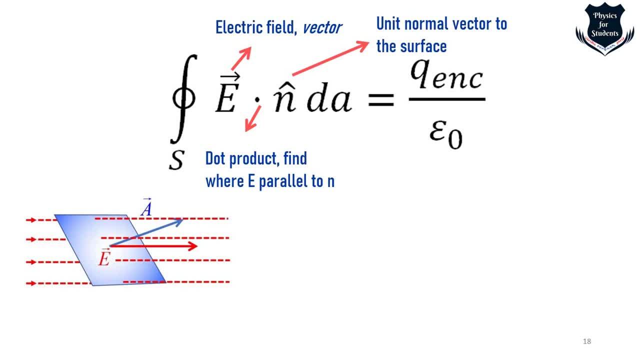 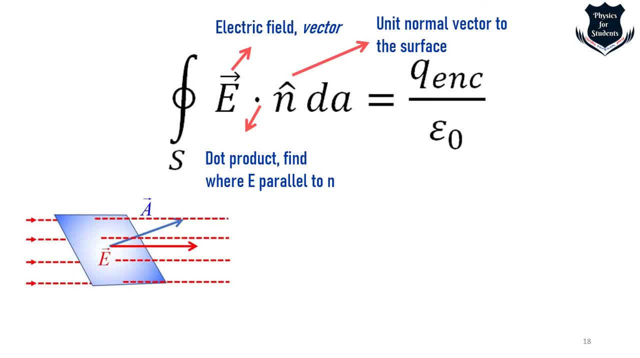 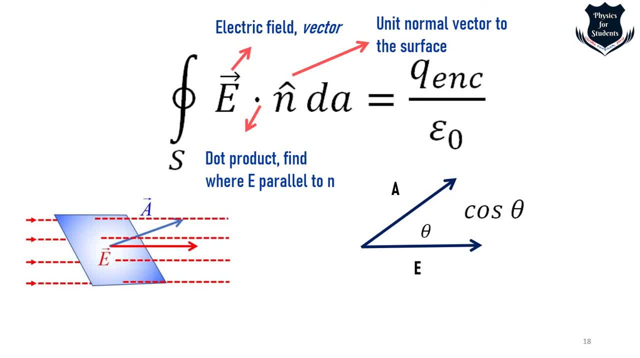 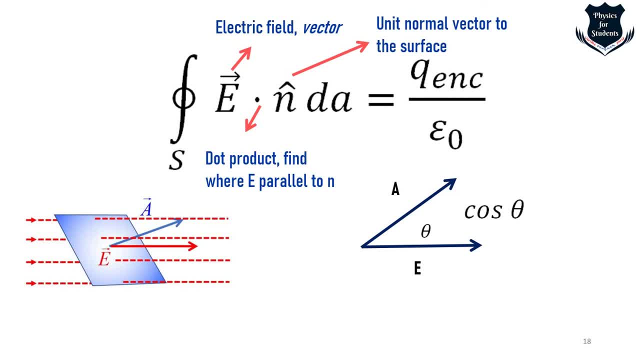 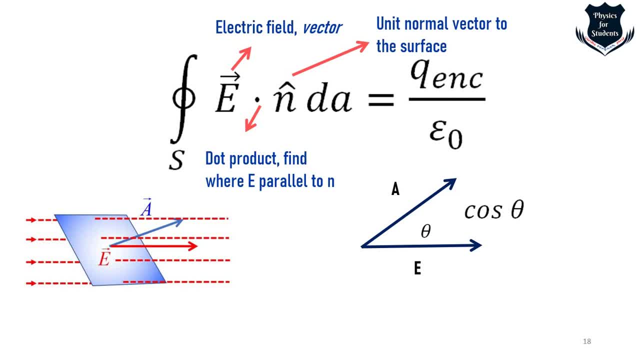 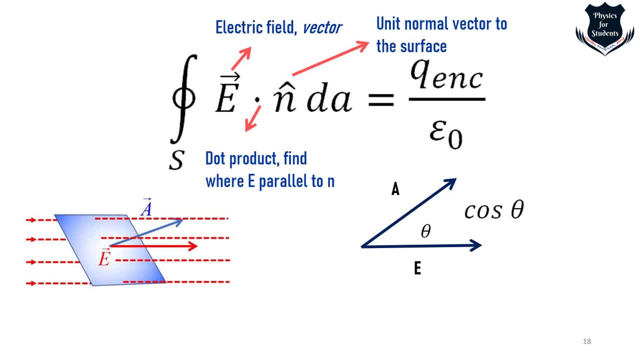 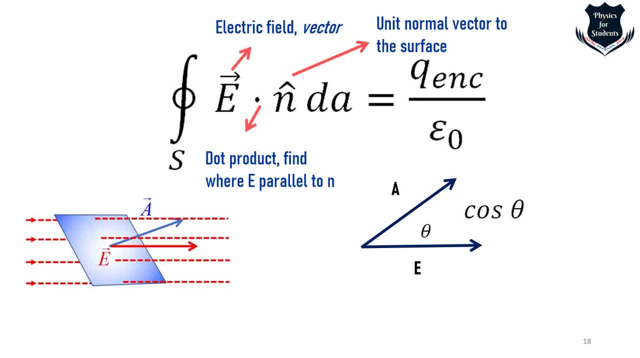 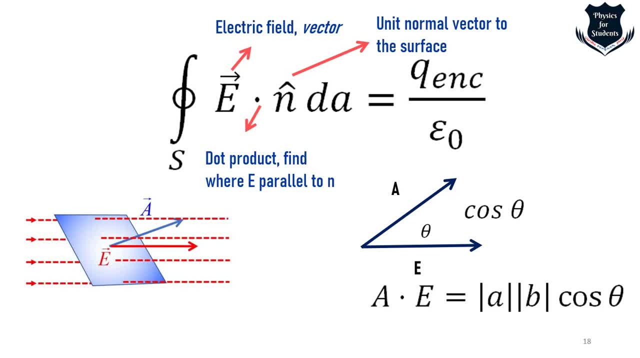 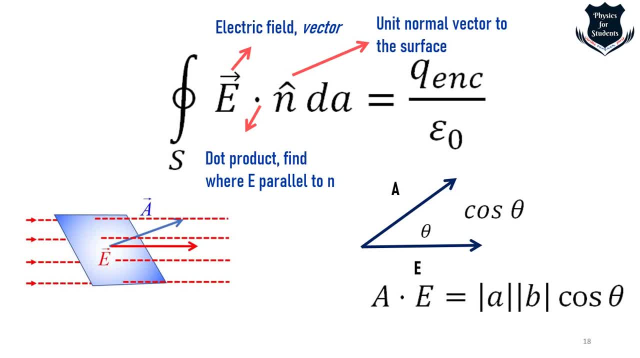 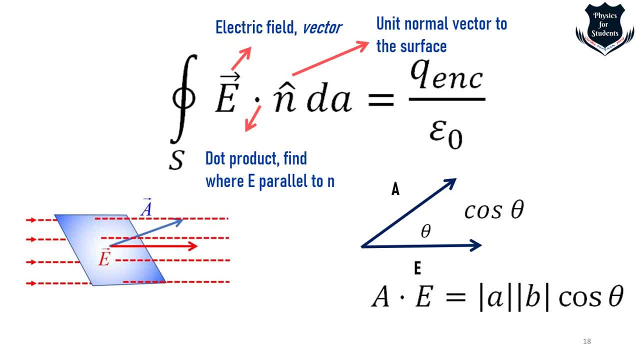 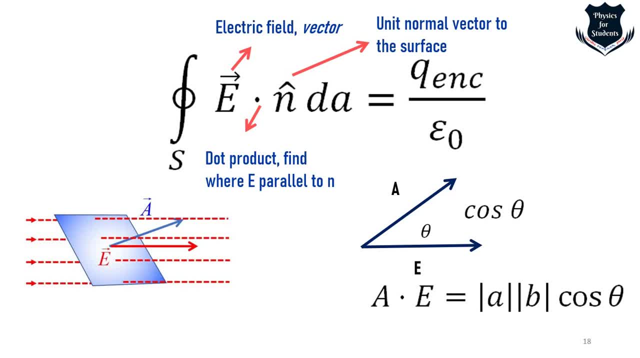 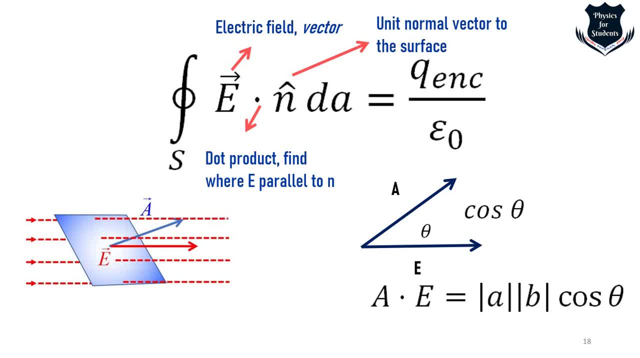 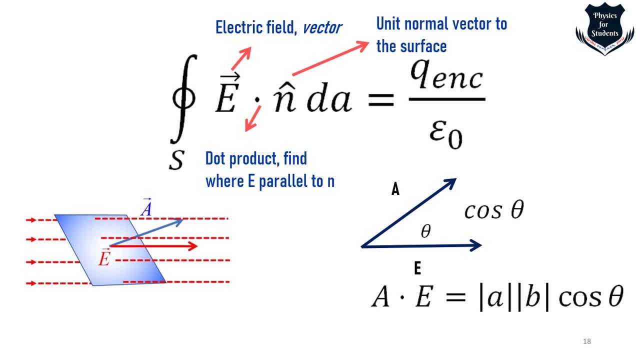 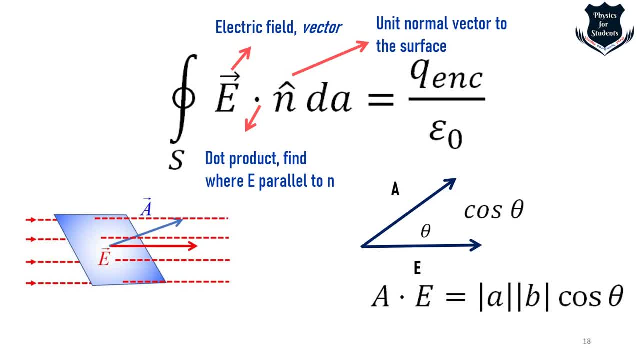 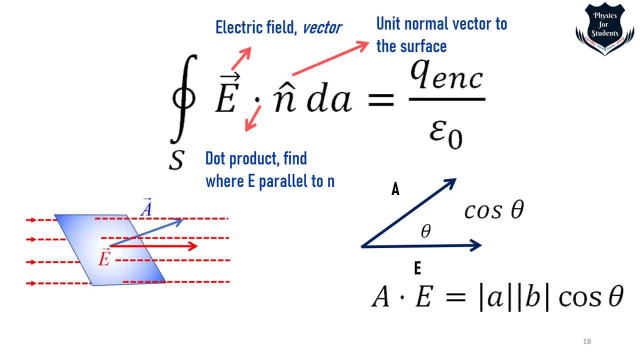 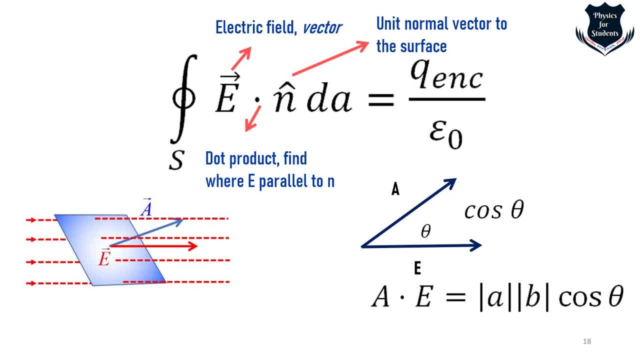 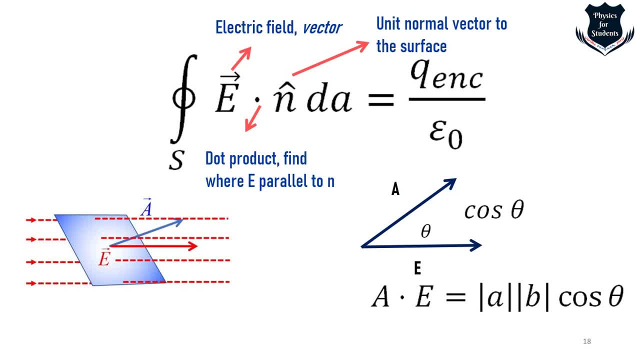 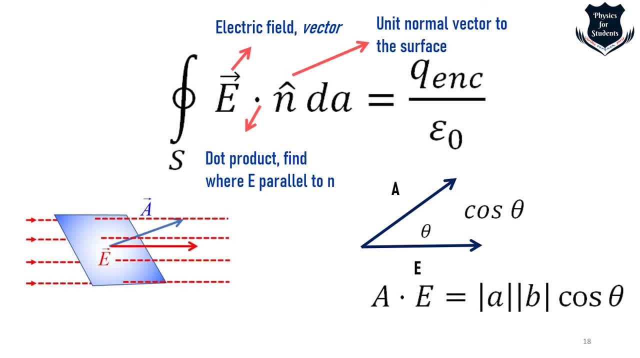 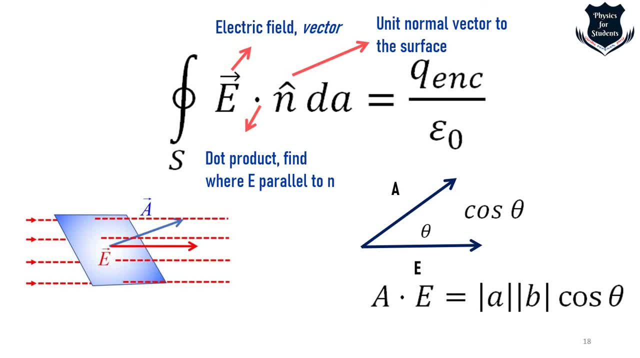 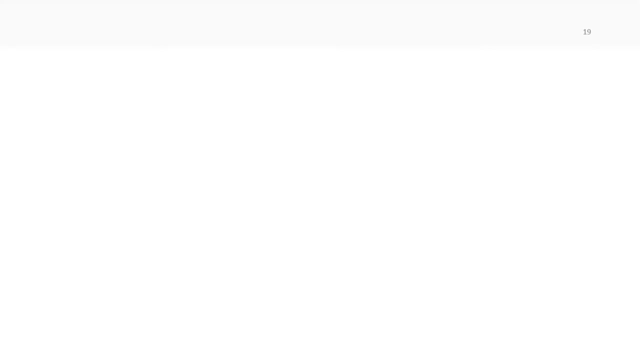 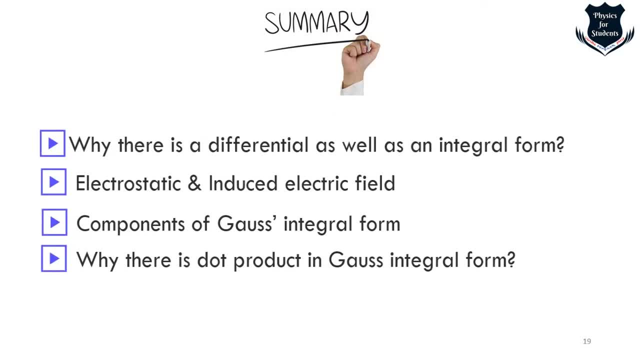 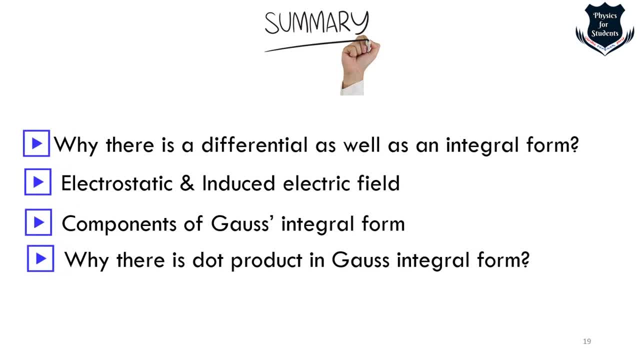 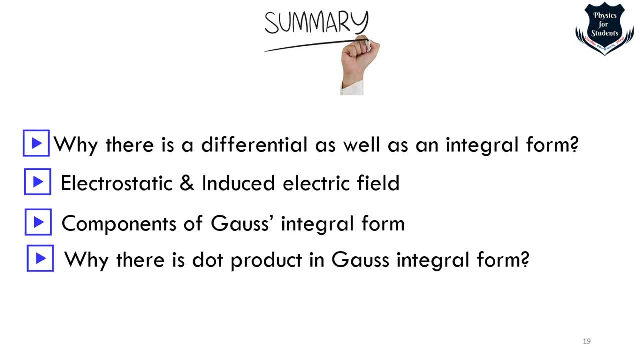 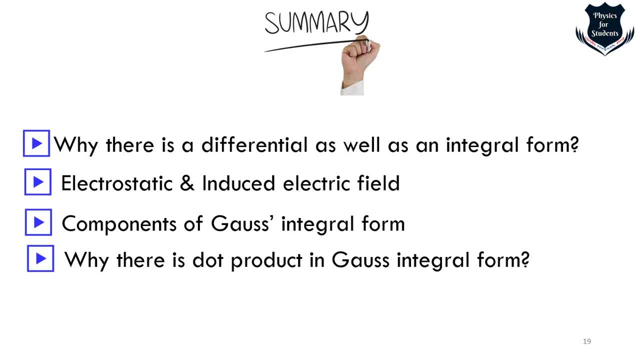 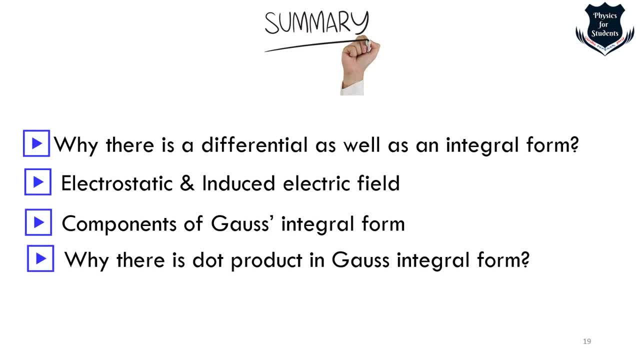 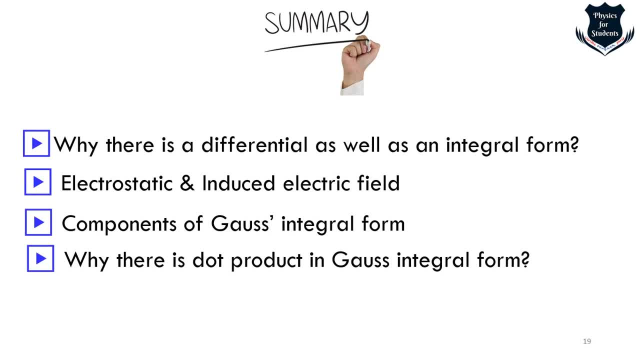 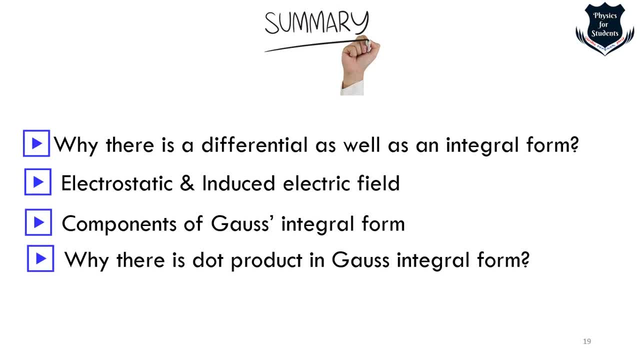 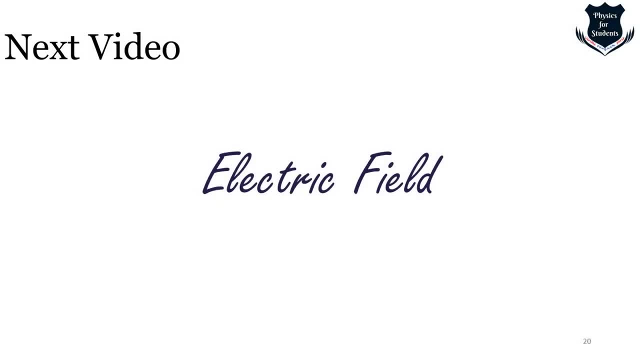 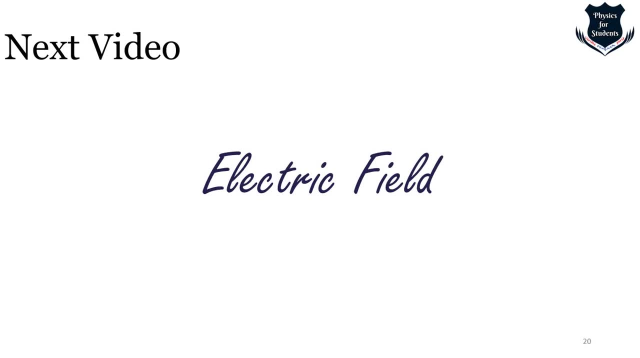